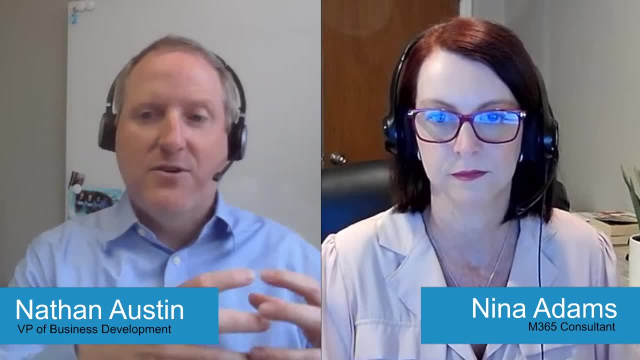 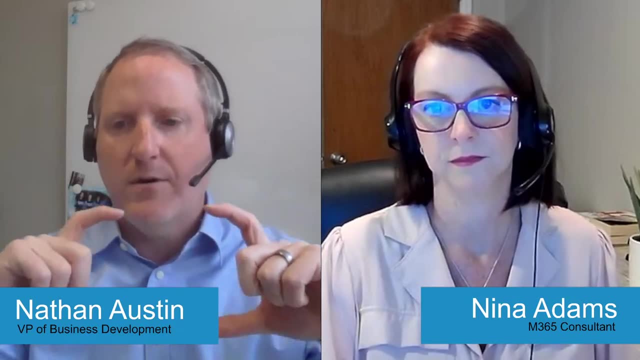 part of that department, like, for instance, we're going to be going through an HR site. This could be a marketing site. This could be an internal IT site, This could be an operational site. This is something that's more designed around what a department head or department might want to use SharePoint. 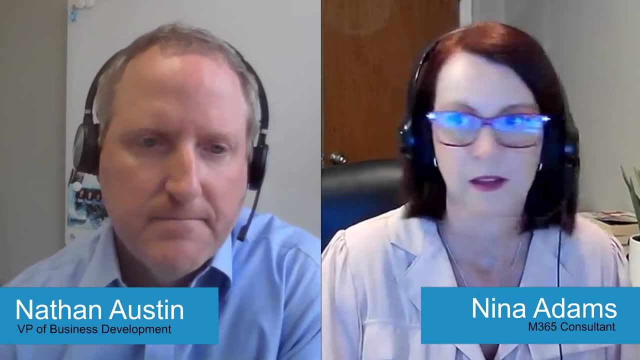 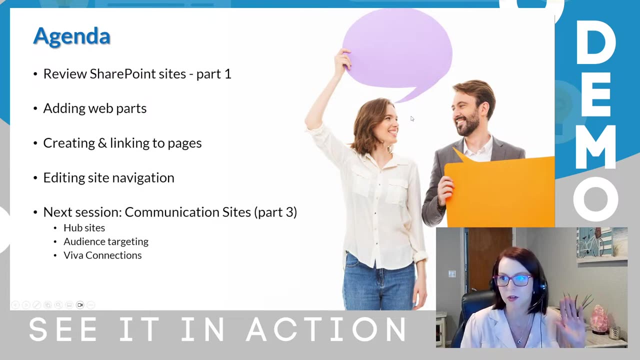 to communicate to the organization. So, with that said, Nina, take it away for Part 8 of the Train the Trainer series. Thanks, Nate. Just a quick look at our agenda for today. quick two or three minutes. i want to review what we did in the last sharepoint session as we started. 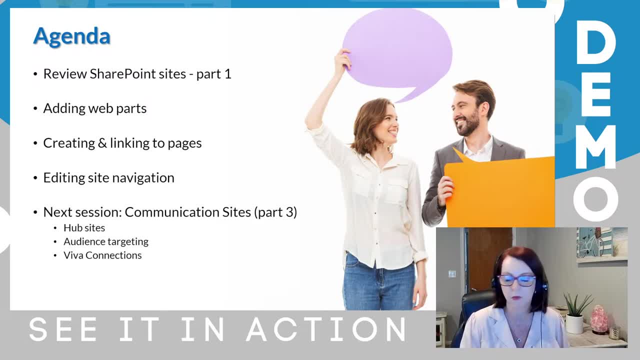 building out that communication site. i want to dig in a little bit more today on some of the web parts, things that i've seen work really well with clients that we work with, and then you know from there, where do i, how do i go about further building this out, so having additional pages, that 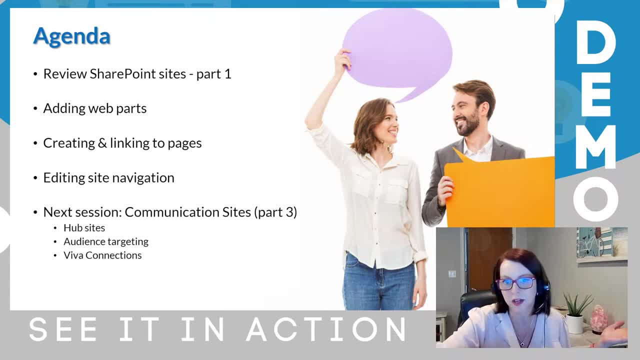 i can potentially link to- and how do i link that to my communication site? where do they live? very importantly, i remember starting out with sharepoint and then creating the page and couldn't get back to it again. i wasn't sure where it was. so very key piece to know there as well. looking at the 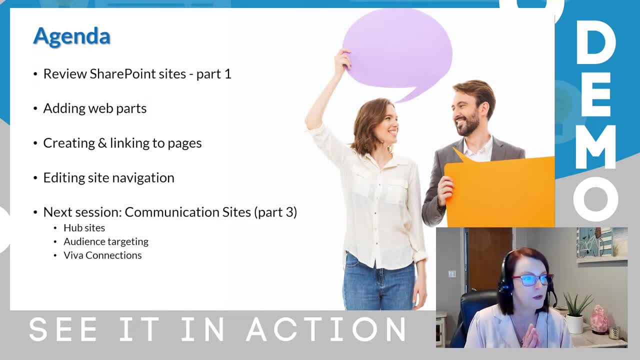 specific site navigation and then for the next session we're going to be putting all of that together. so where now we're very much focused in on one department, like hr- again, as nate said, it could be marketing, it could be it, but in the next session we're going to look at how do we actually 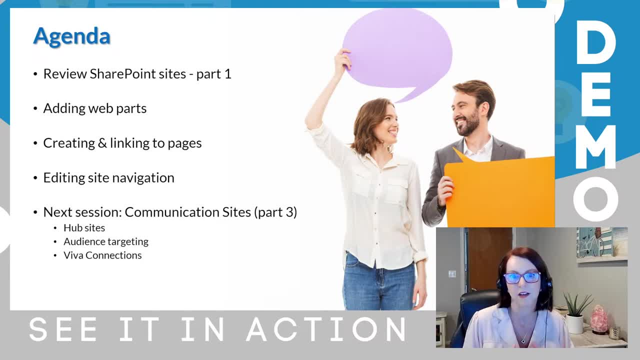 pull all of those you Sites together using a hub site and how do we make the navigation really easy to use? how do we make it intuitive? how do we do things like audience targeting? so we want to make sure that specific links are relevant to people. we don't want them to be clicking on a link and then they get an. 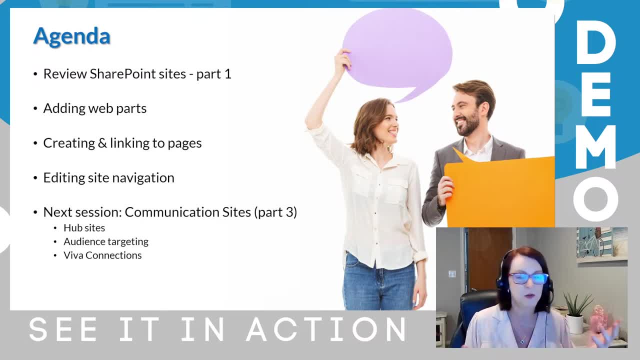 access, denied notice or something to that effect, and then also leveraging viva connections so that i can actually start tying my sharepoint site in with microsoft teams. we've really found that the easier we can make it for people to get this, the easier we can make it for people to get this. 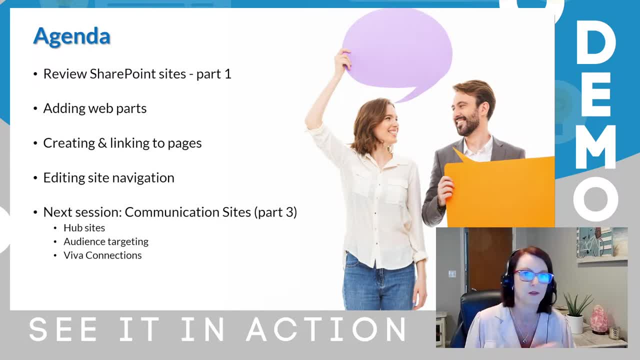 there, the more likely they are to use it and to adopt it. but if they have to leave teams, and then, you know, go, hunt down sharepoint and then the navigation isn't intuitive, those are all things that are very typically roadblocks to people adopting some of this. so, with that being said, i 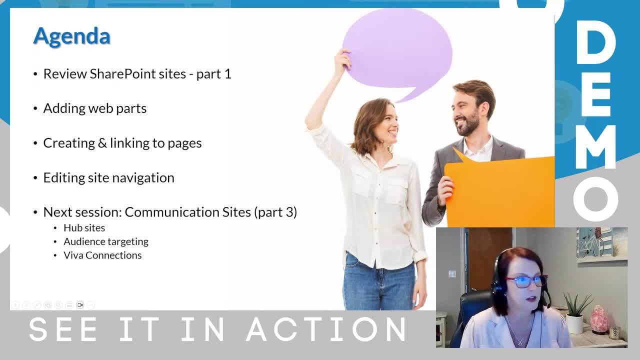 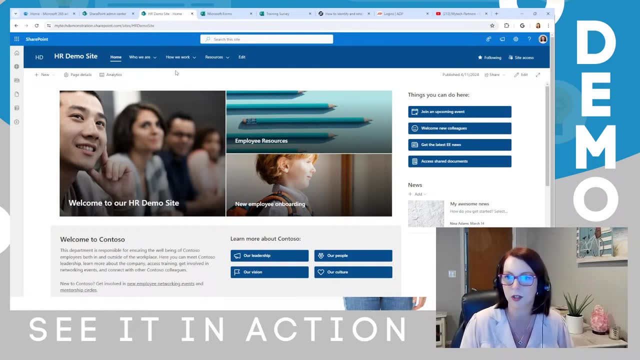 am going to hop into our sharepoint site that we had created the last time. so this: in this particular use case, we were building out a communication site for human resources, just really quickly. again, the difference between a team site, which is really more for internal use, if you're thinking of. 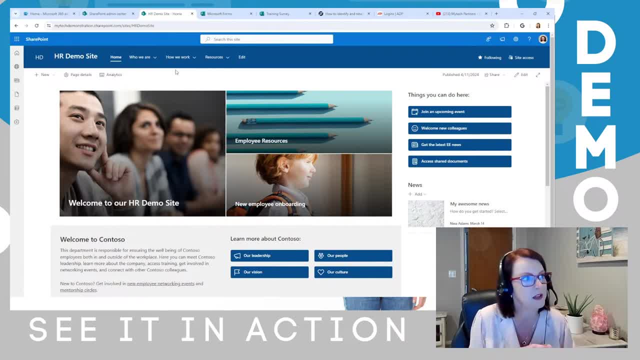 microsoft teams, some of those groups that maybe you participate in, whereas what we're building here is where we want to share some of those final published versions of documents, things like policies and procedures, employee handbooks- that type of thing we don't really want people to be. 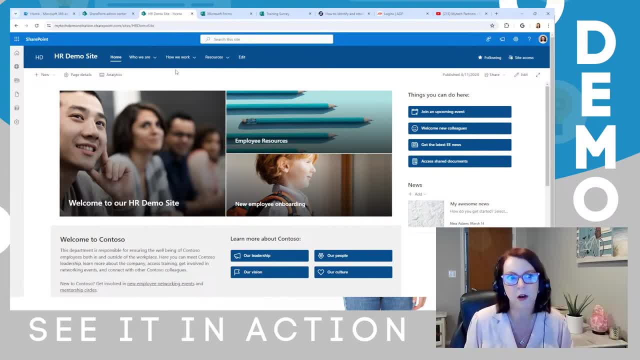 changing them or editing them. we want to make them a read-only copy but we do want to make it easily available across the organization, which is where the communication site is located, and we want to share some of those final published versions of documents communication site comes in. so in our last session we created this using one of the out of the box. 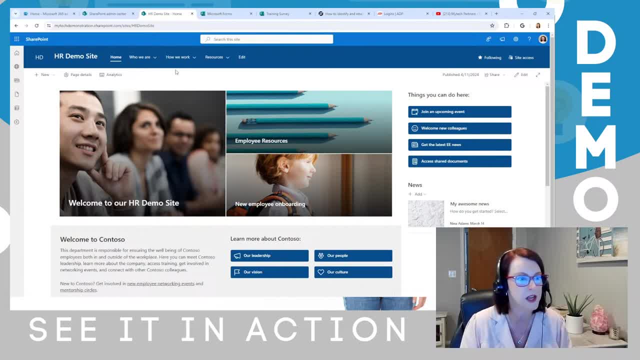 templates. so there are a variety of templates there to choose from, and i showed you some very basic changes that we could make by editing the page. so again there's. as a site owner, you have two edit buttons here, so one on the right hand side where you would edit the page and one here. 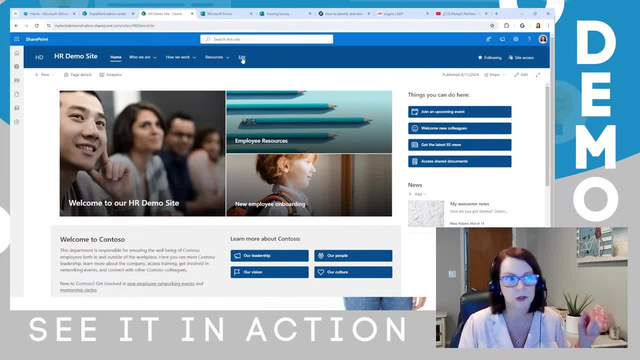 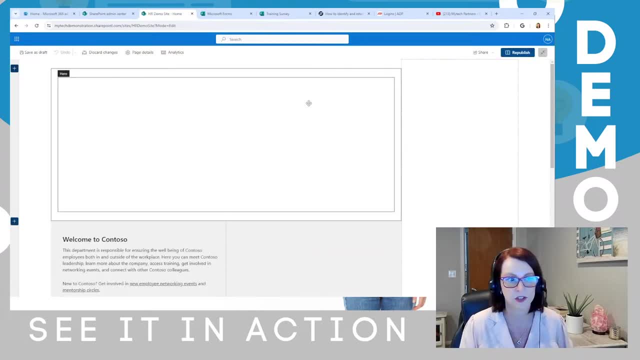 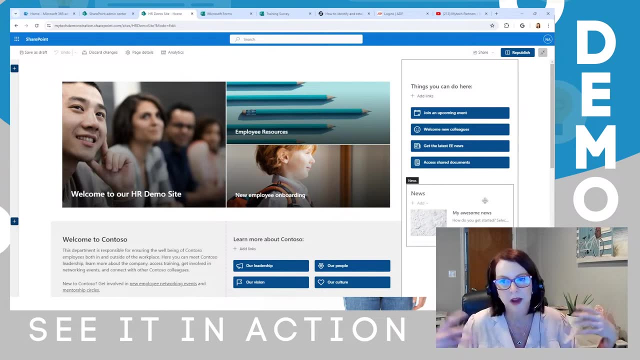 top middle where you would edit the navigation. so we will look at that in just a minute. so again, if i hit this edit button over here, we spoke about having different sections on the page, so we added in a right section here where we kind of discussed really maximizing some of that page real estate by implementing a right-hand. 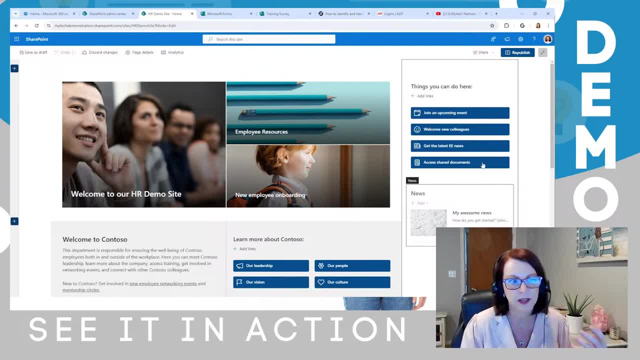 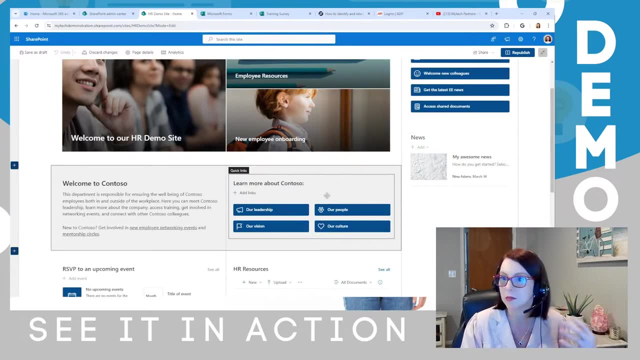 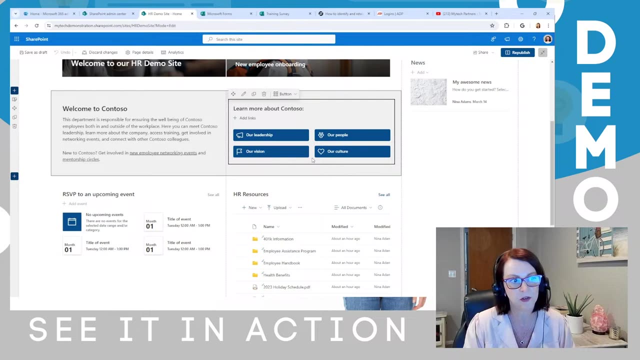 column and creating some web parts. in there we have quick links. we have a news web pod. you'll notice as i float the cursor over, the little border pops up so these can be moved around so i could easily click and drag. i can add new web parts by. if i float the cursor here, a little plus sign pops up and from there i'd be able. 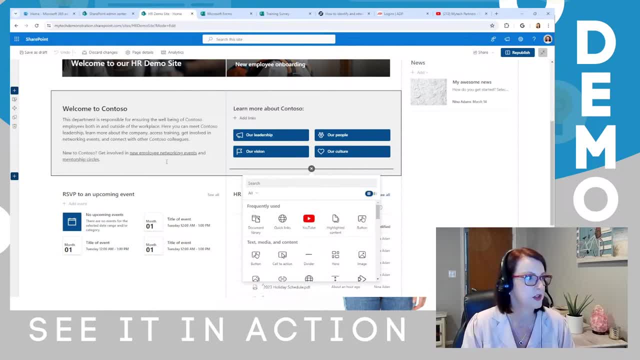 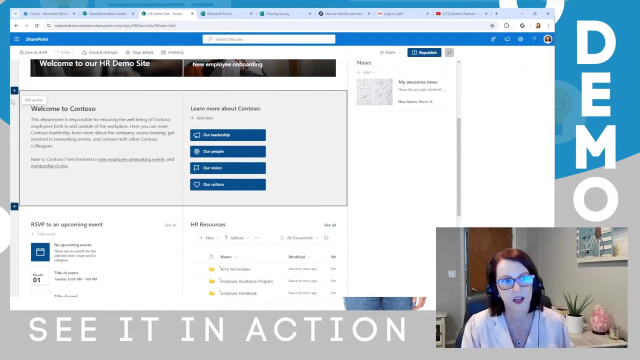 to add in additional web parts. we also discussed adding in sections. so this is kind of adding in sections onto your page to add additional content, and this can be done by clicking on the little blue plus here on the left hand side. also here you could edit the section. so if i click on edit, 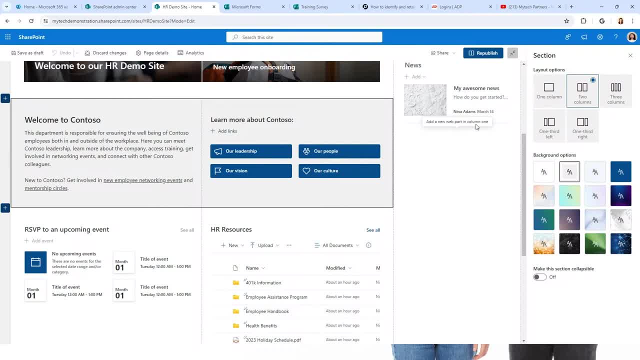 i can change things like how many columns i have and what background colors i would want to utilize. i just noticed here, nate, they've added in some new background colors, which is always fun, as you're doing demos, to notice that new things were added since the last session, so that's always. 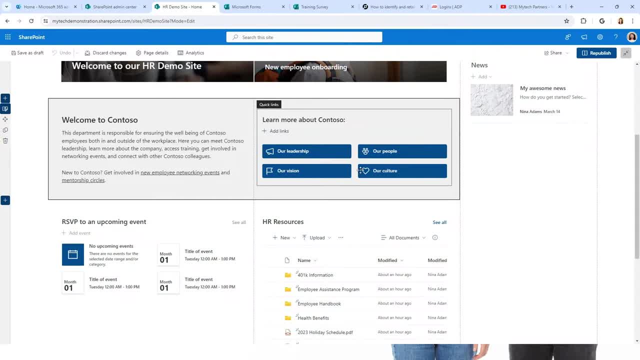 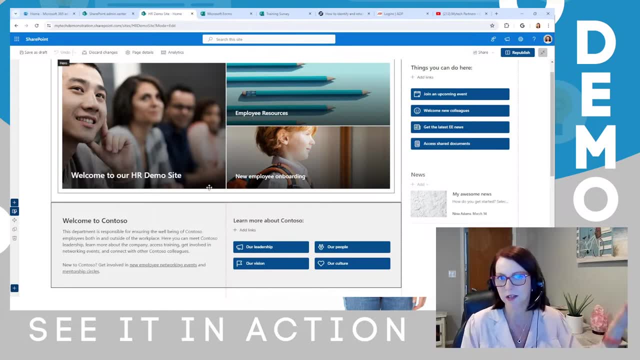 interesting to see. all right. so that's kind of what we covered in the last session. one of the concepts that we talked about was kind of best practice on the layout. i always recommend that you try to keep it as uncluttered as possible, especially the landing page. think of it as a 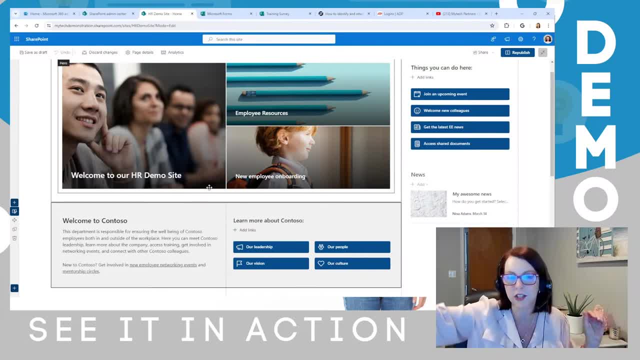 dashboard and from there you can add in some new package colors and you can add in some new. there we would want people to link to other additional pages or additional resources. Having too much content or having it go down too far down the page, people are much less likely to. 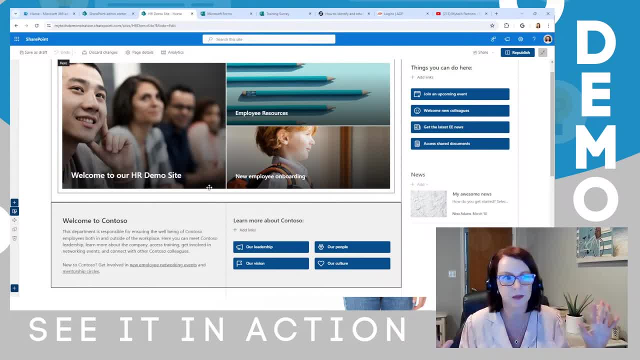 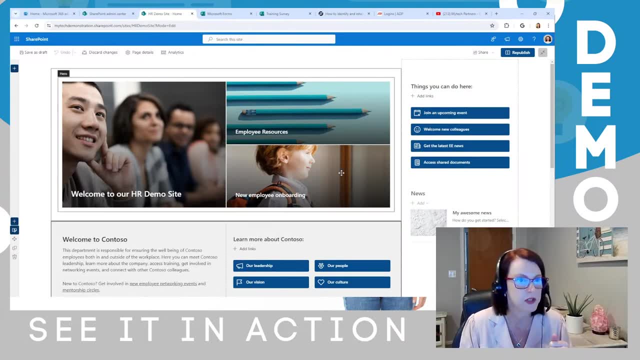 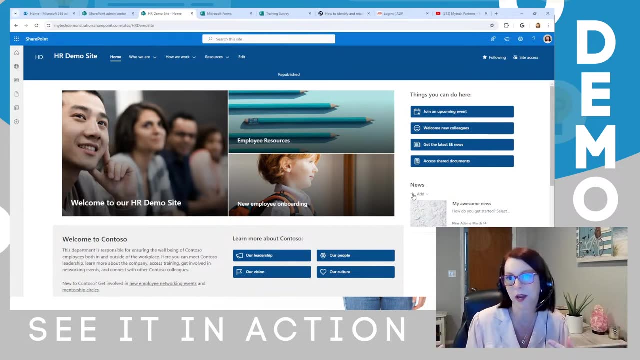 actually go hunt for stuff in my experience, So I try to keep it as clean and uncluttered as possible. All right, So in this particular example, I'm just going to hit the republish button And I want to show you how you, from here, can add in additional pages and then link to those. 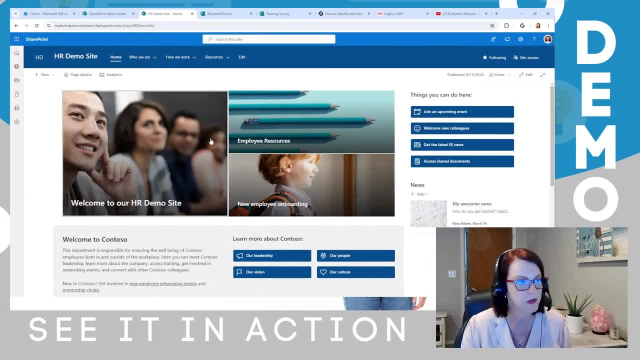 So in our hero web part, which is this visual web part here at the top of the page, we have two tiles that we created in the last session, but we didn't actually link it to anything. One is something to link to employee resources and one is a tile that would link to 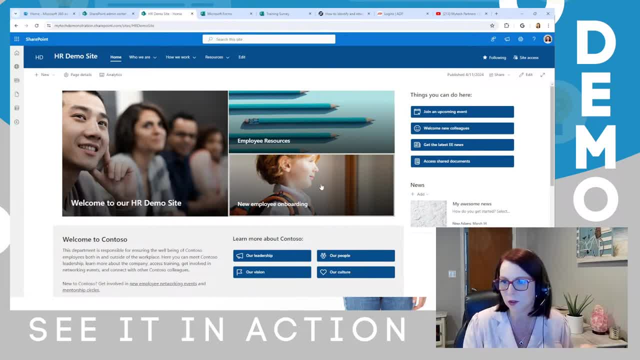 onboarding. This is particularly useful, I've noticed as we do work with clients. As a new employee, you kind of don't have to do a lot of work to link to those. You're a little lost when you first start and trying to find all the different policies and 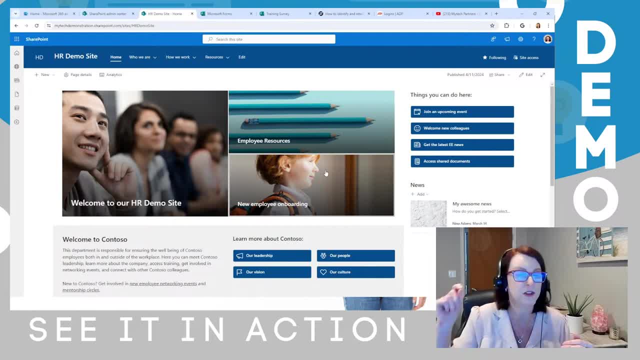 procedures and handbooks and things like that, or maybe a checklist of things that you need to do within the first 30 days. 60 days, 90 days can be a little daunting for new employees, So one recommendation that I make is to actually have a page set up or an area set up in your site. 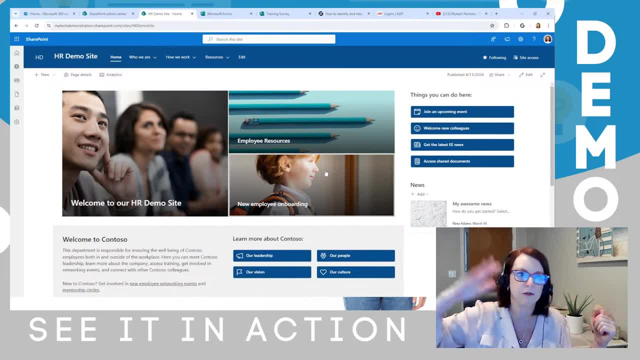 where a new employee can go and find a checklist of resources, videos, training, you know, checklist- Whatever that looks like in your organization. it just makes it so much easier for them if they can find everything they need in one spot. So we're going to create a page to do exactly that. 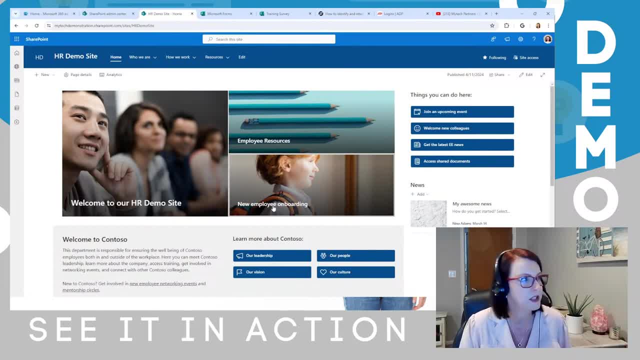 I'm going to do one for new employee onboarding And to do that I head over here top left. There's a new button and you'll notice if I click on that there's a couple of different things that I can actually create from here. 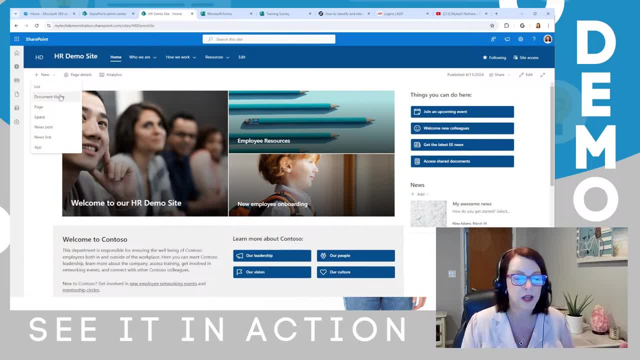 So I can do lists. I can create an additional document library. Remember that you do get a default document library. You can create an additional document library with the site that you've created, But if you wanted to, you could create additional ones. 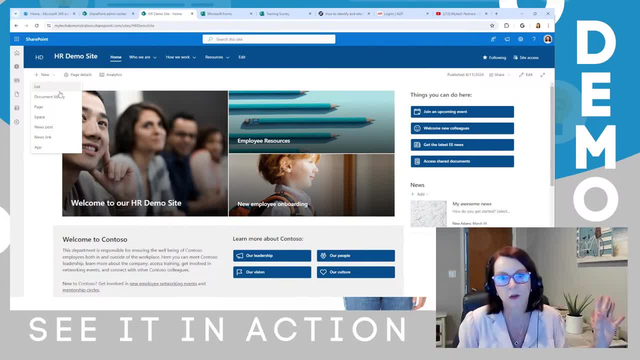 So maybe you had two very separate categories of information and you wanted them to be in different document libraries or maybe had different metadata. We spoke about this in the document collaboration discussion And you wanted those to look very different. You can create additional ones. 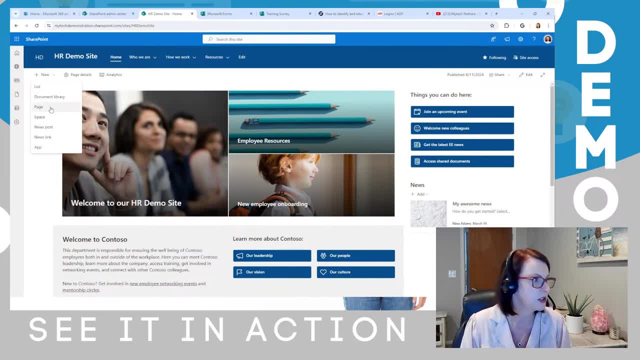 And the third option here is to create a page. So that's what I'm going to do right now: I'm going to go and create a new page. A couple of tips, The templates to pick from. I just usually just go with the easy one. 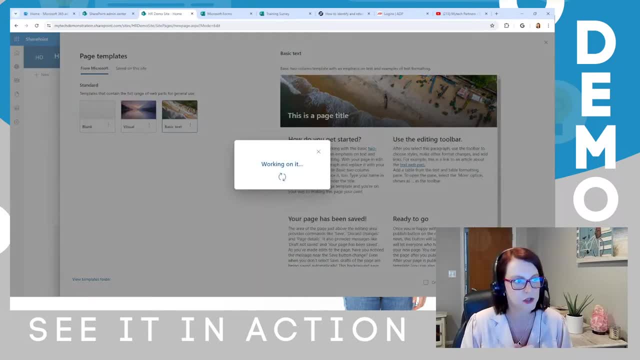 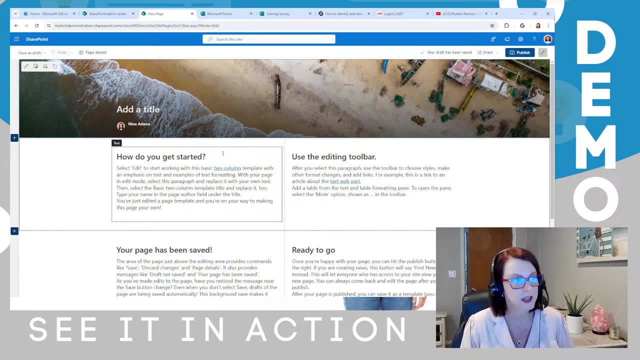 the basic text and click on create page. And very similar to how we actually edited the site. I can go and make edits to this page by simply clicking on it Again. I can add in additional web parts here. I can just kind of like working in a Word or PowerPoint document. 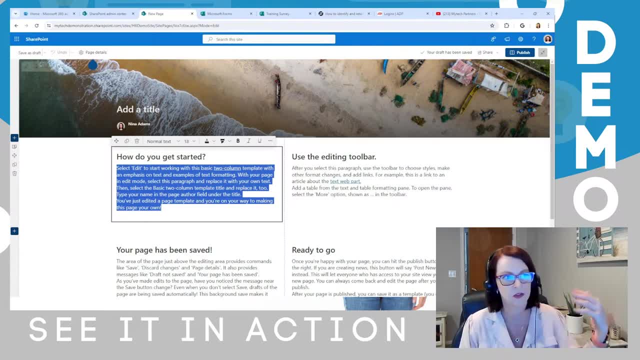 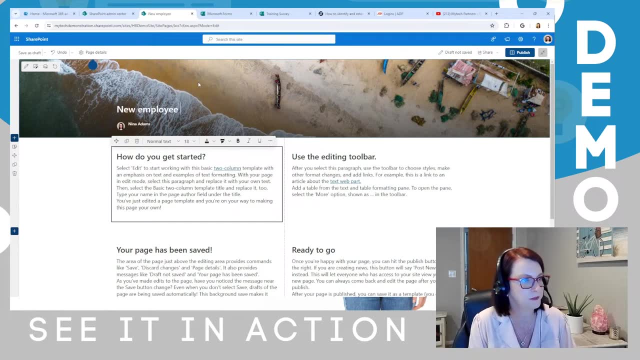 I can go and edit the text pretty easily, And the same with the heading. So let's start off here at the top and we're going to say new employee and I'm going to say, oops, onboarding Top left. here I can change the image. 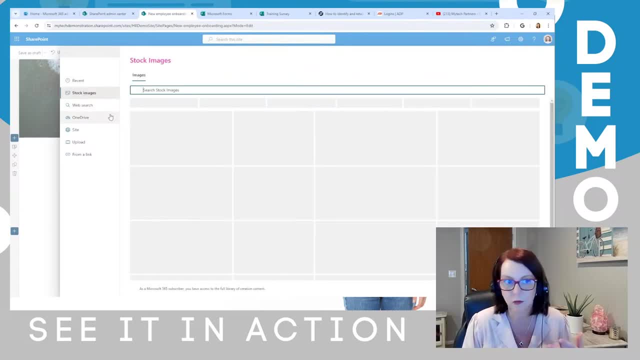 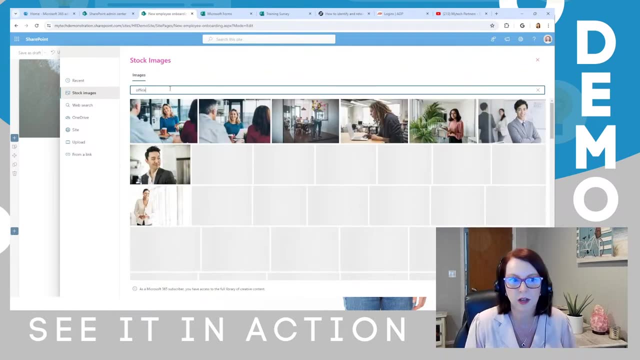 So again, we have quite a number of stock images that come with our 365 subscription. I'm going to, and then you can search. So if I say office, I can get quite a few resources that are related to office and people in an office. 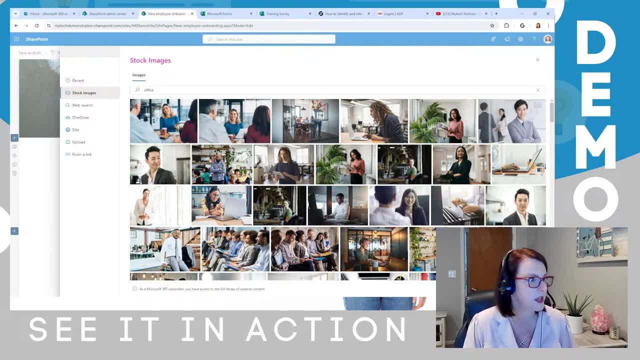 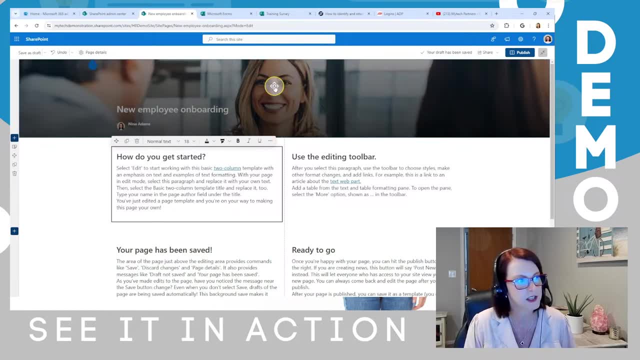 So I'm just going to pick a random picture over there With this little button here, the set image focal point, I can move it up and down, So I can position it very nicely pretty easily. So again, no code required, nothing. you know no developer skills or anything like that. 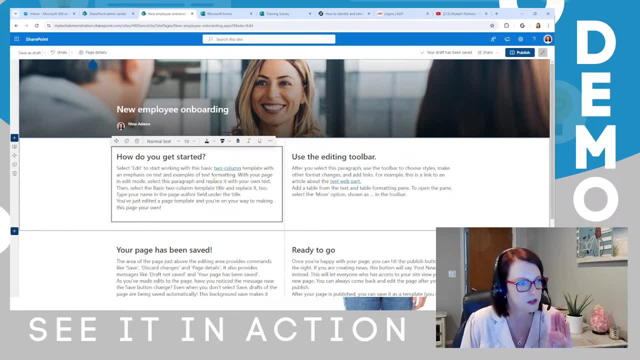 It's actually pretty easy and pretty intuitive. So just to make this a little bit easier, I'm going to remove this little web part, this text web part, If I click on it. excuse me, click on the trash. can I do want to give them very quick access into our HR document. 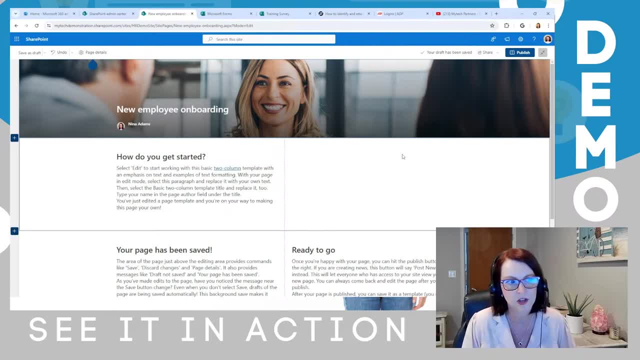 So I'm going to pull in our document library, kind of create a shortcut. So I'm going to do that for them there. So if I float the cursor, click on the plus, I can either search through here- You'll see it is at the top of my list- or I could just type in document library. 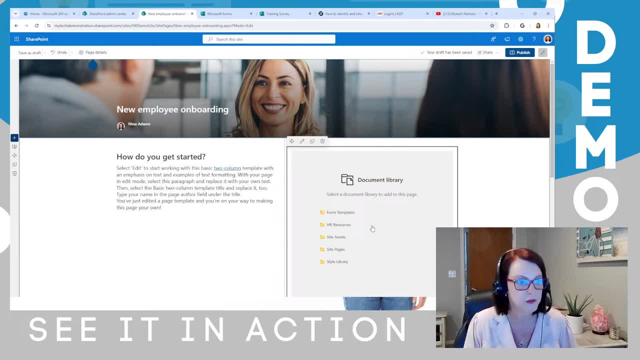 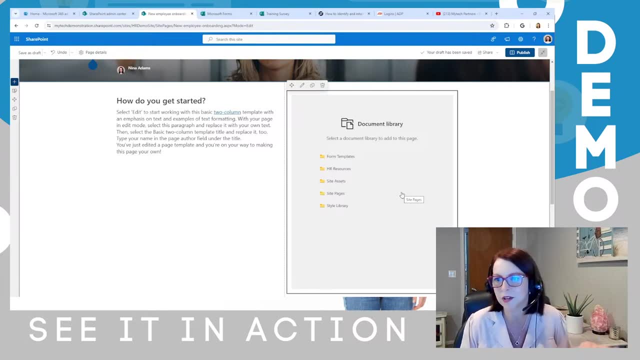 So that's what I'm going to do. So these are the document libraries that are currently attached to my site, Just as a side note. style library, site pages, site assets: those are kind of default libraries where all of your photographs, logos, 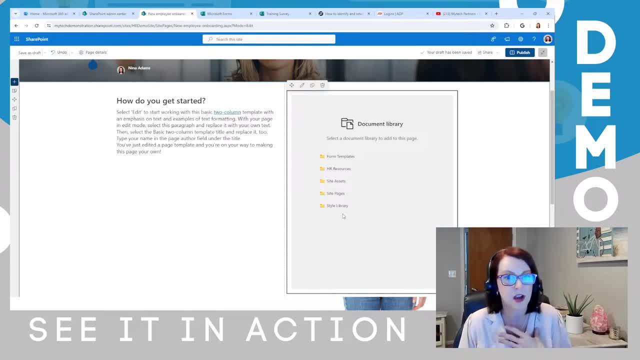 and all of those templates kind of reside, So I'm not going to do too much. but I have my own document library called HR resources, So I'm going to click on that and there we go. really nice and easy It's. I always see it as multiple ways to get to the same thing. 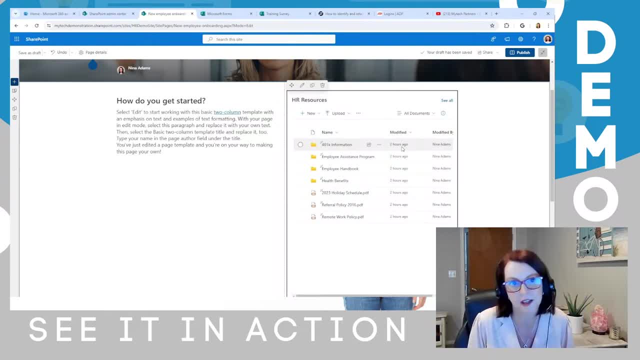 So, yeah, there's still only one document library, but I'm just making it a lot more easy and accessible for new employees to find. So this sectioning here is a little squished. So if I go here to the left-hand side I can say edit section. 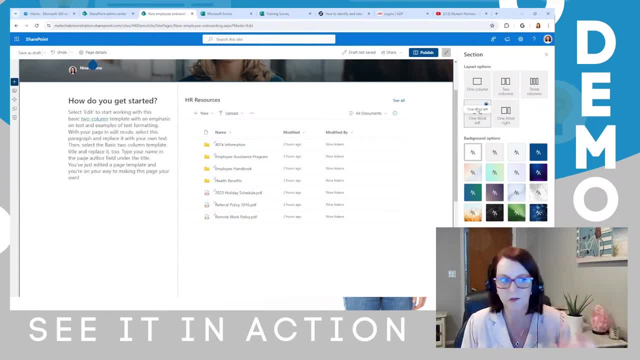 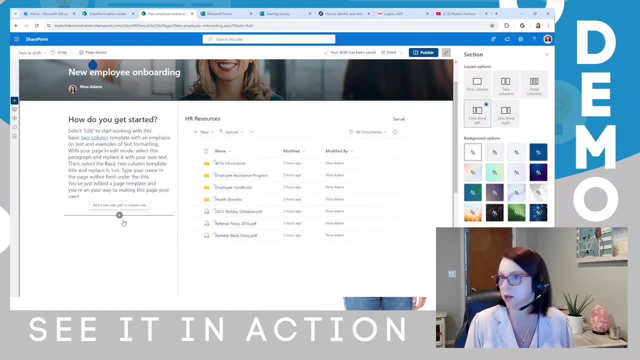 and maybe I would rather make this a one-time section, But I'm going to go to one-third left just to kind of have that display a little bit better. Alright, and then below here I might want to put in a video. 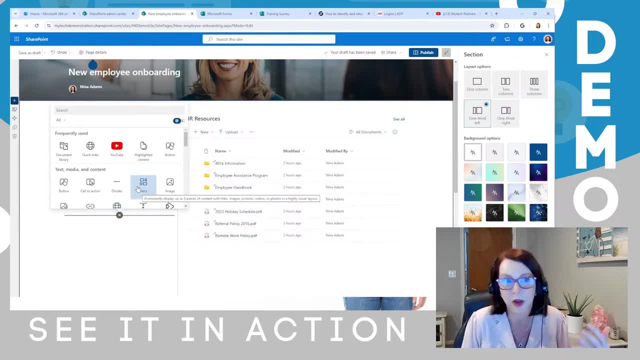 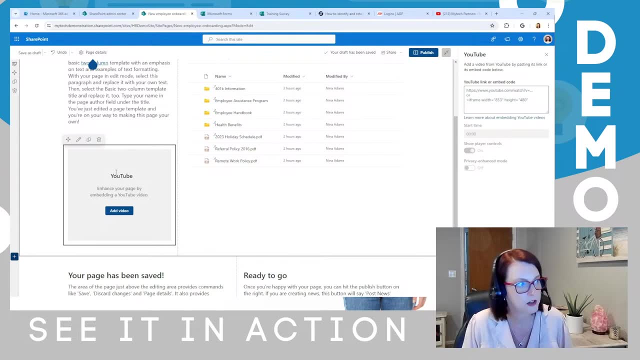 Let's say I want to put in a little YouTube video that has some training or a welcome video. So I'm going to choose YouTube right there And remember that with every web part that I click on there's a little pencil icon And with that I will see the properties on the right fly out panel. 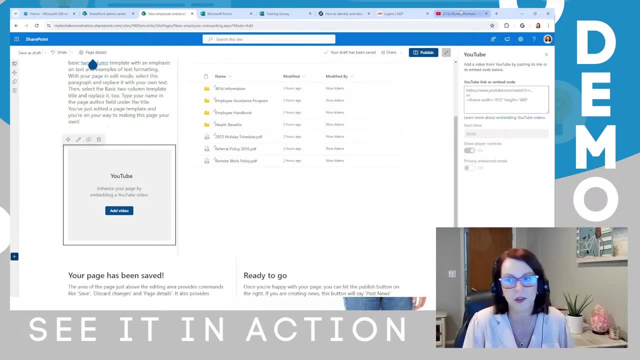 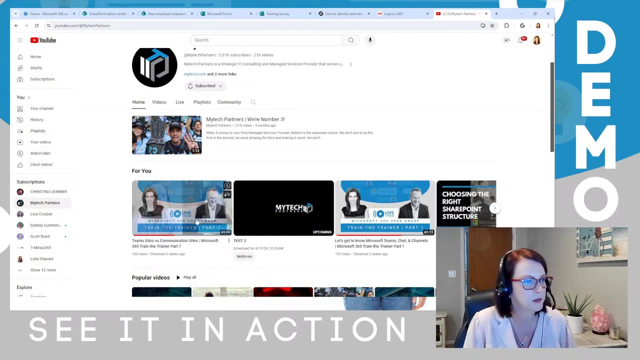 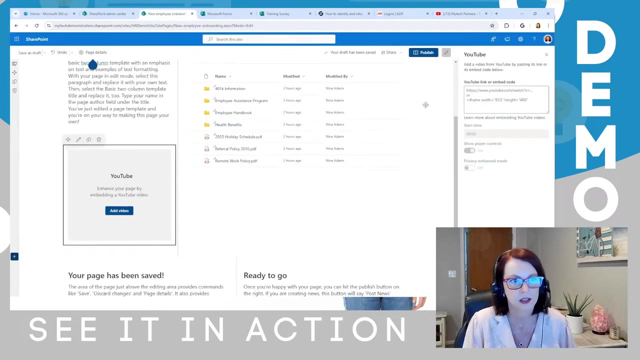 So here it's looking for YouTube code. So I'm just going to head over here to our My Tools Tech Partners YouTube channel And let's say, here's a video in here that I wanted them to see. So I'm going to right click on there, copy that URL And here in the YouTube code just paste the. 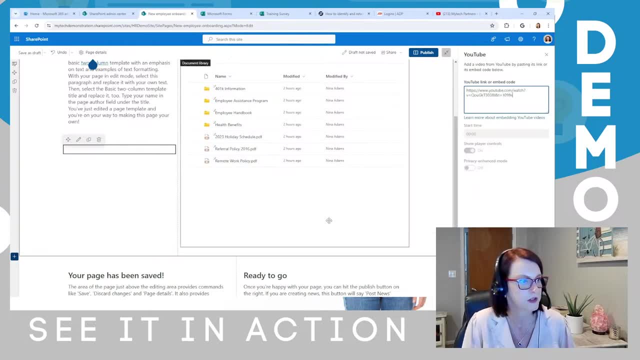 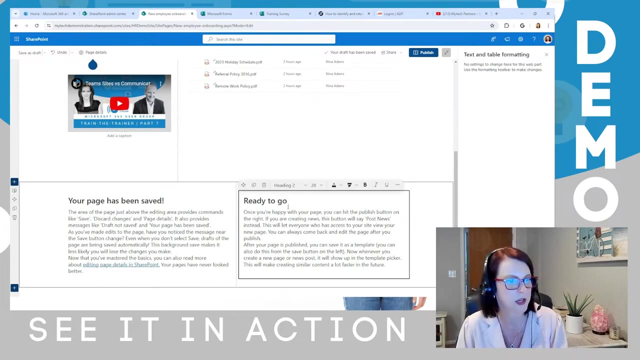 code in there, All right, And you'll see a little preview will pop up there. There we go Really easy to do So any other resources or useful training videos that you wanted to link in there really easily, And let's say, down here we wanted to create a checklist. So I'm just going to just 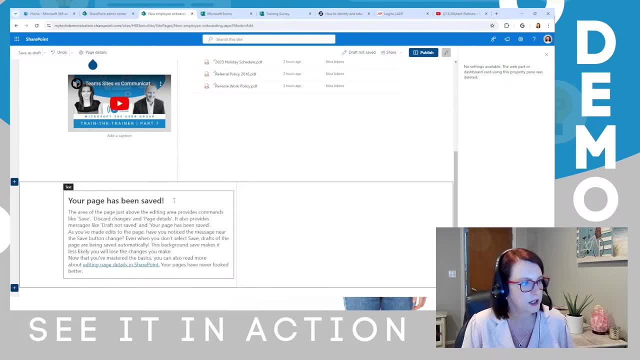 delete this really quickly. So this is going to be a new employee onboarding checklist, And this could be in any format. Maybe you already have an existing Excel document or maybe you're utilizing a SharePoint list. We've found that that works really well, But for this example, I'm just going 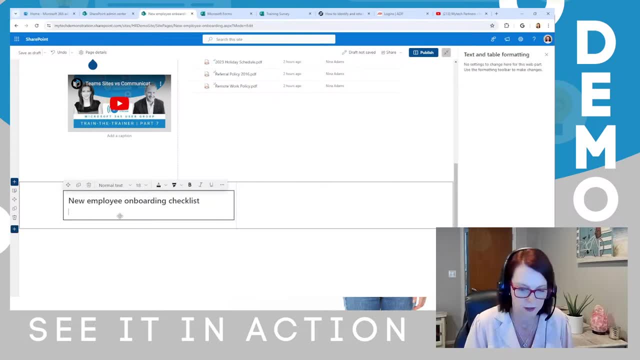 to put in a few bullets. And while you're doing that, Nina, I'll just kind of chime in on, like if you're a department head right now and you're thinking, gosh, this feels overwhelming And why would I be doing this versus. 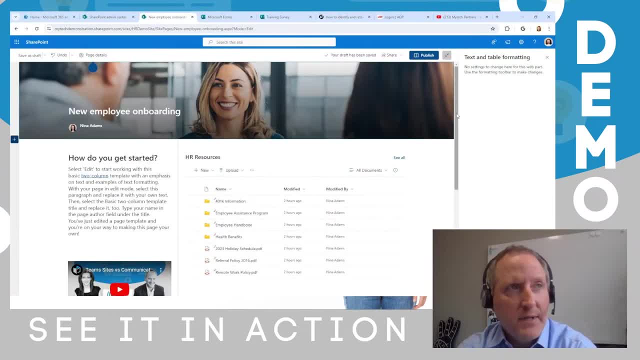 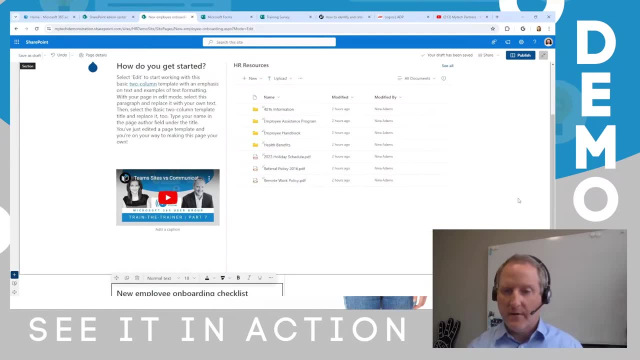 somebody in IT And I think, conceptually, that it doesn't have to be a department head. In fact, some department heads might not be the right technically savvy ones to do this. They might feel uncomfortable doing it. So maybe you find a chance to do that And I think that's a good. 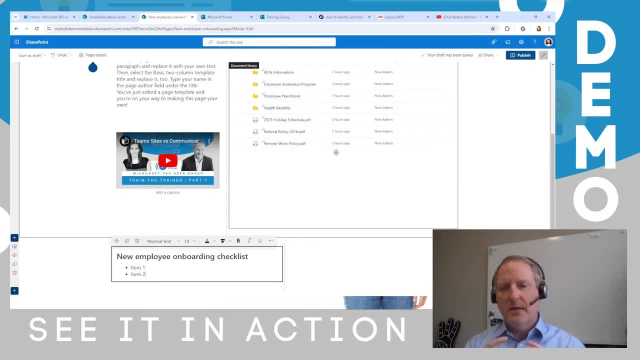 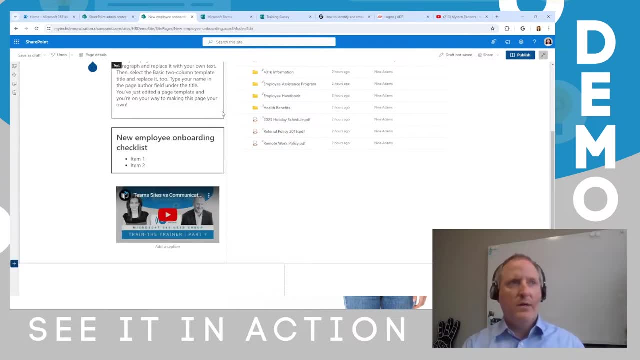 way to do that, And I think that's a good way to do that, And I think that's a good way to do that. But the theory around this and the reason why we're focusing initially on a SharePoint site that might be considered for a department like HR, is that that way you can delegate responsibility. 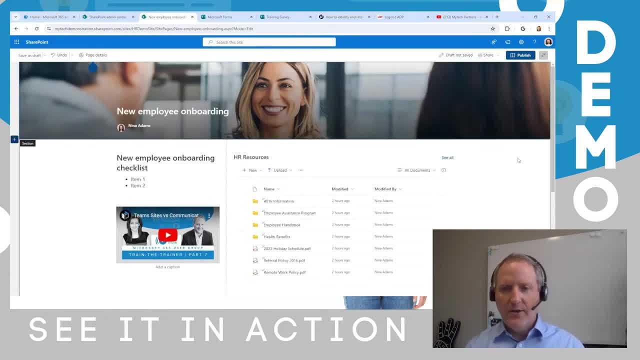 to people in the HR department to communicate things about HR. You don't have to go to IT to post something. You don't have to go to marketing to post something. You don't have to have a marketing, IT, operations and HR site because different people might want to have different. 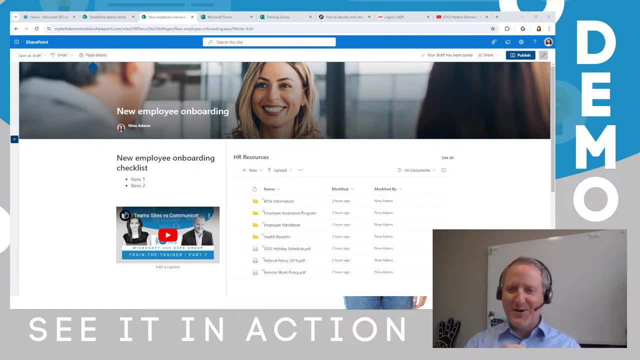 layouts. So you're not going to create conflicts as far as how different people might want to try to manage your site. So you're not going to create conflicts as far as how different people might want to manage their own pages and their own communication. So the concept here- and I think it's I really do. 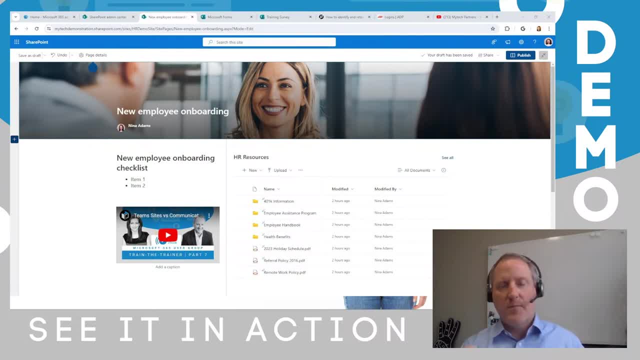 appreciate how Microsoft has built this out is that you as a department, whether you're the department head or a champion or power user inside of that department- can really have the authority to be able to communicate things relative to your department out to the organization and design it. 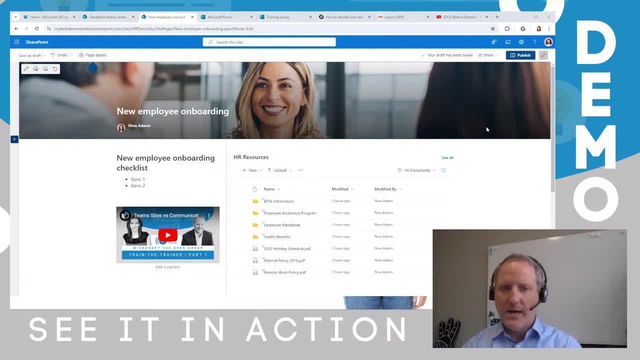 in a way that you feel is the most intuitive for your audience, And so, as opposed to having one site where everyone manages and everyone can have the opportunity to design their own thing, you could kind of do that. So there's definitely some training going on, but I think what Nina has shown- and sorry Nina, I want to 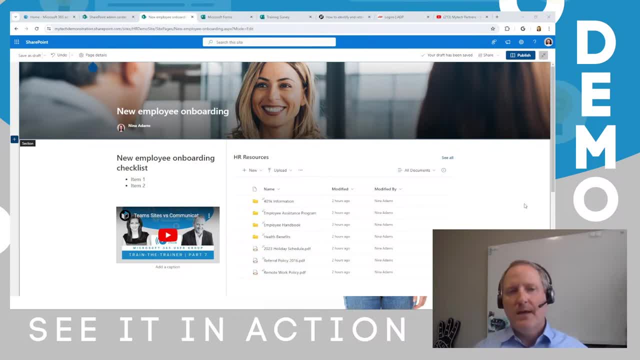 buy you time to write some of that stuff. but what Nina's showing is that there's a lot of pieces to it, but when you break it down to the individual parts, each individual part is basically the same as far as how you click the. 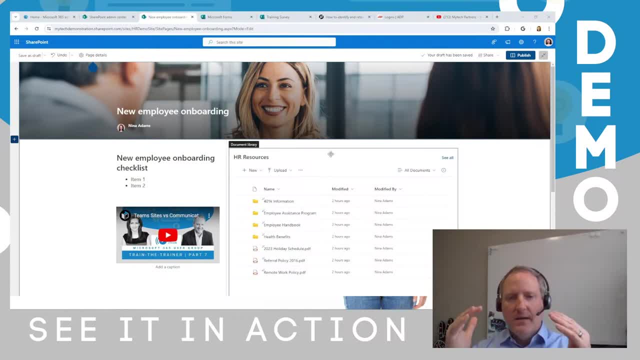 little edit button and you can pull in different pieces And so just trying to lower the anxiety if you're not a technical person where you're really about, like if I'm an HR department head, but I don't feel comfortable with this stuff. That's why we're trying to go through this at an individual site level to hopefully help cascade the concept that we feel has been. 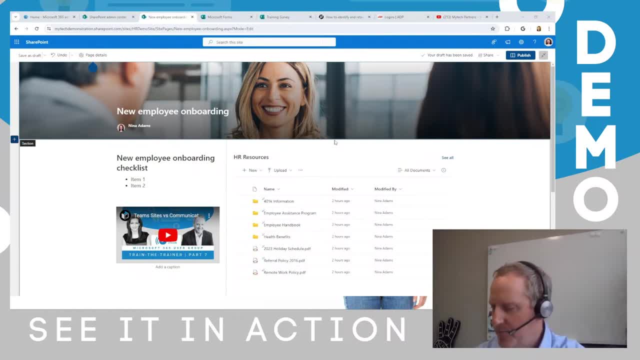 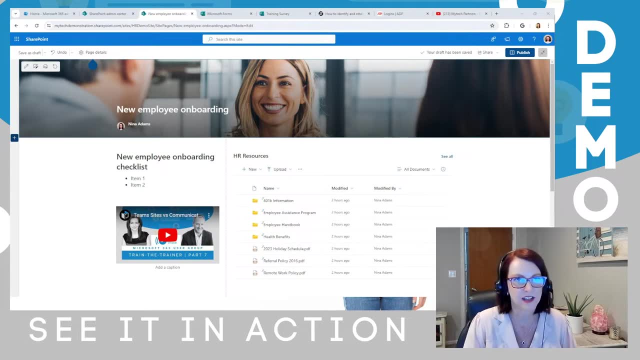 successful across a lot of clients we've worked with. Sorry, Nina, hopefully that's put a little extra context as you're navigating through your agenda. Perfect, Thank you. Yeah, and that kind of distributed responsibility is a model that I found with clients works really well. 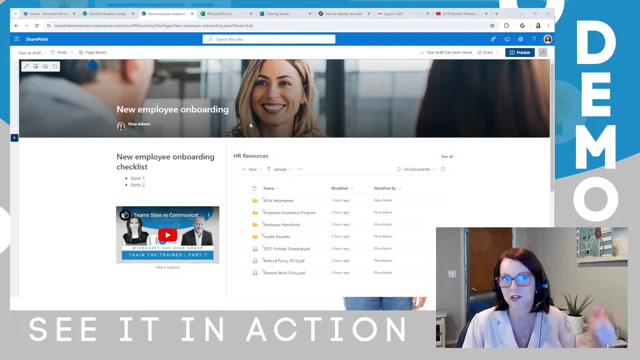 I will probably just touch on the permissions, just again, just those three items. So the out of the box permissions were really your site owners, and then your members or contributors, and then really the larger organization or those visitors or read only permissions. And what works really well is that maybe as an HR, the head of HR 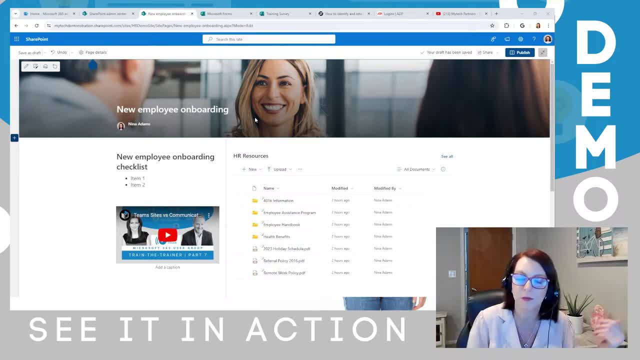 maybe you are a site owner but you have one or two people that are helping to kind of keep that content up to date. Obviously, stale content means that people won't come back, But you know, having people to help You are not, as you mentioned, having to go through an IT department or put in a ticket to get something as silly as content up to date just seems to work. 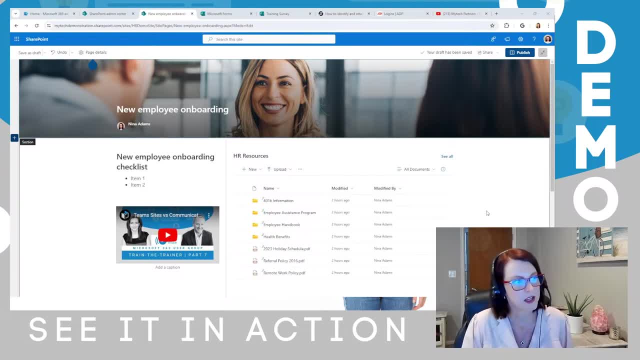 really really well. All right, So this is a very basic employee onboarding page, but at least it just shows you how you can pull in things like a document library, a video, a text. I'll show you in a minute how to add some additional stuff in there as well. 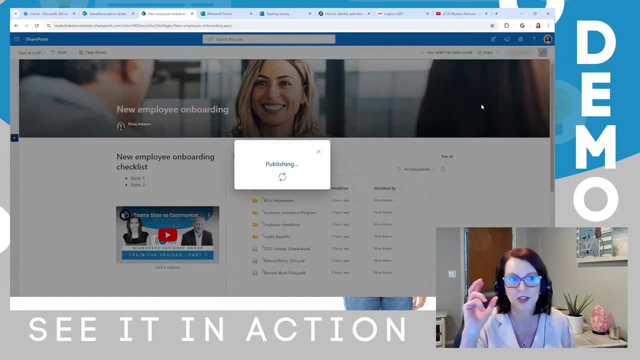 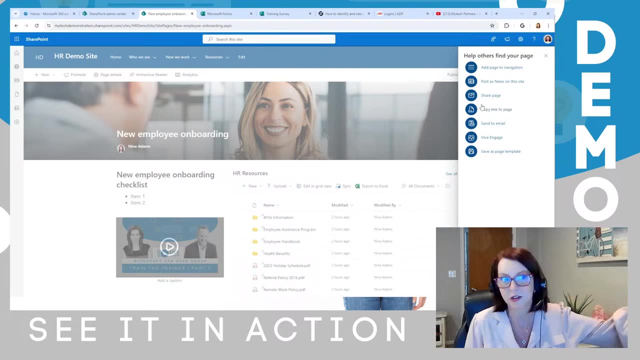 So I'm going to go ahead and hit the publish button And, very importantly, I want you to see what pops up the minute I do that. So there's a couple of different options. Once the page is published, I can add it to the navigation if I wanted to. 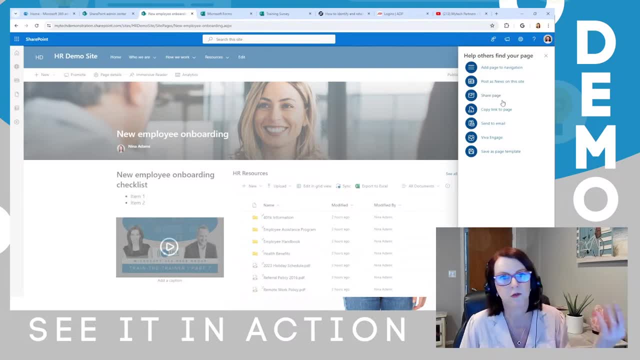 I could share the page via email or, you know, via Teams chat. So a couple of different options there on what I could do for this particular example, Remember I want to link it to that initial hero web part on the main page. 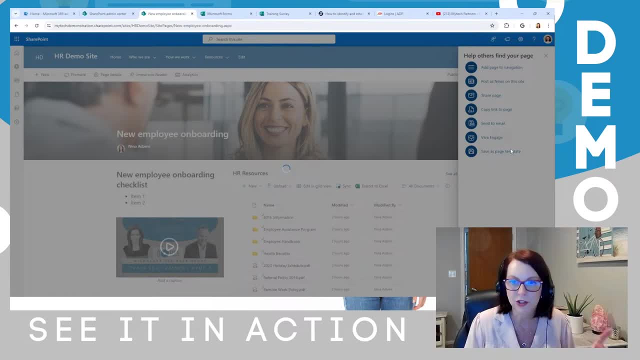 So I'm going to say copy link to page, but I will show you where that page now resides because, as I said earlier, this has happened to me many times. So I'm going to say copy link to page, but I will show you where that page now resides because, as I said earlier, this has happened to me many times. So I'm going to say copy link to page, but I will show you where that page now resides because, as I said earlier, this has happened to me many times. So I'm going to say copy link to page, but I will show you where that page now resides because, as I said earlier, this has happened to me many times. 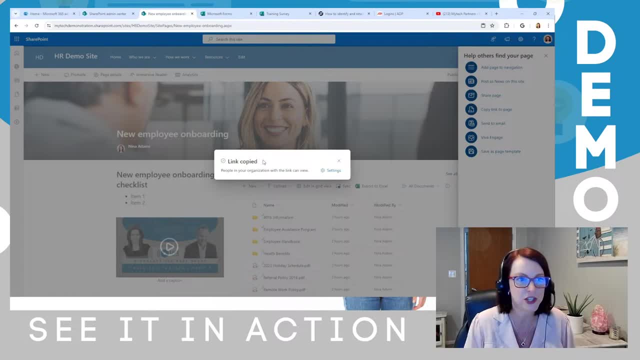 Especially on my. you know, starting out on my SharePoint journey, I would create the page, publish it, forget to copy the link and then navigate away and then not know how to get back to it again. So I will show that in just a minute. 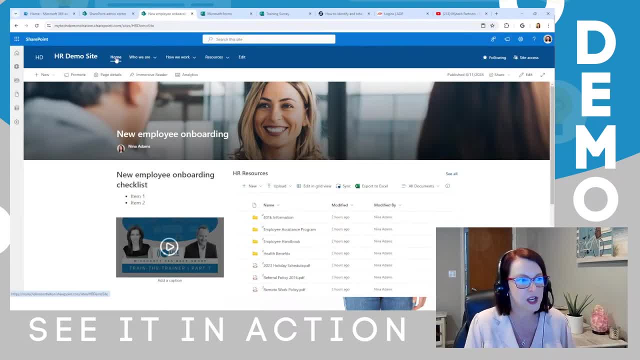 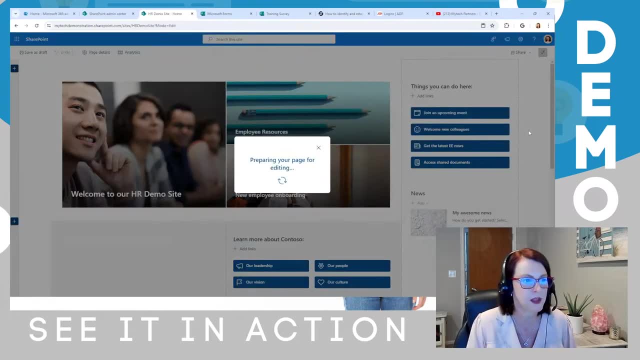 All right, so we've copied the link. I'm going to go back to the home page And now I want to link it up to the new employee onboarding tile. So I'm going to hit the edit button. I'm going to click on that tile. 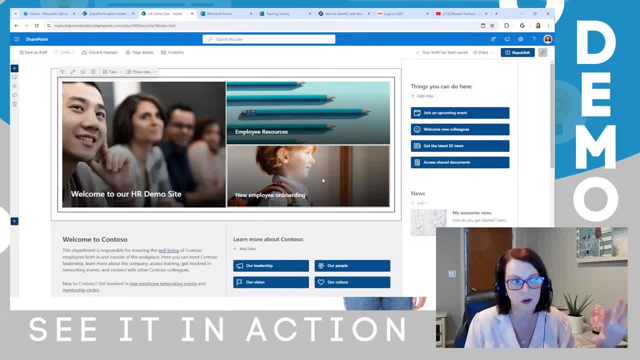 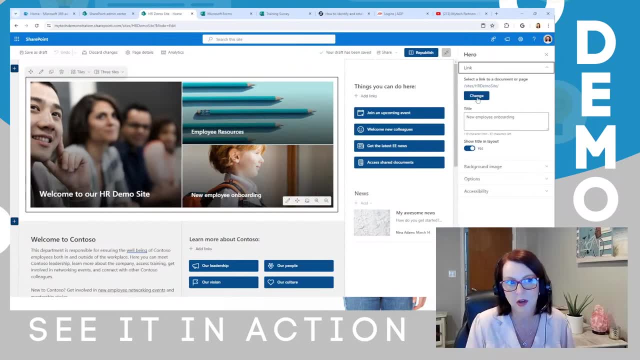 You may have to click twice, Because once selects the whole Euroweb part and the second click will actually click on the tile, Click on the little pencil And right at the top there you'll see at the moment it's linked to just the site itself. 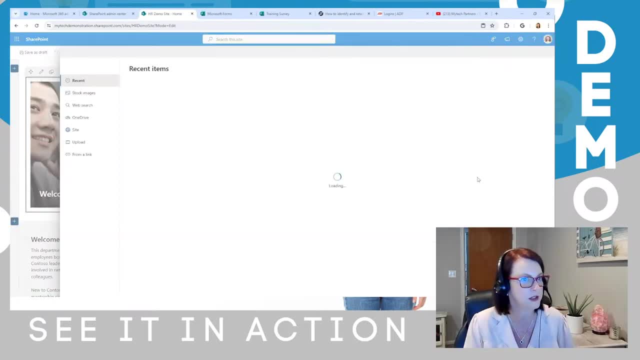 So I want to actually change that to link to the new page that I created On the left-hand side. click from a link And paste in the URL that I just copied when I published And click on add, And I'm going to go ahead and say republish. 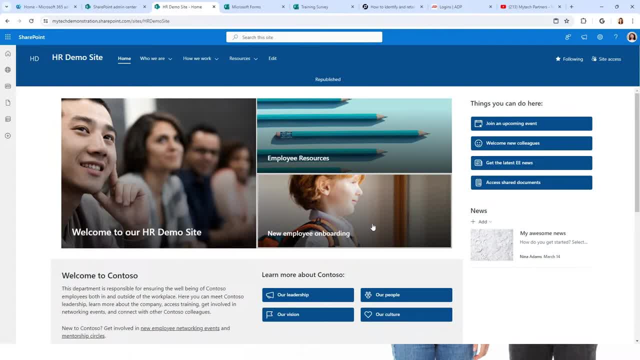 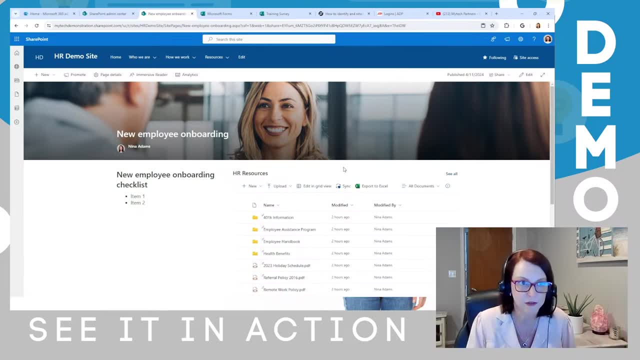 And let's just test that it works. Always good to do So. if I click new employee onboarding, it will take me to the new employee onboarding page. All right, so quickly. where does this all live? So top right here, little gear icon which takes me to my settings. 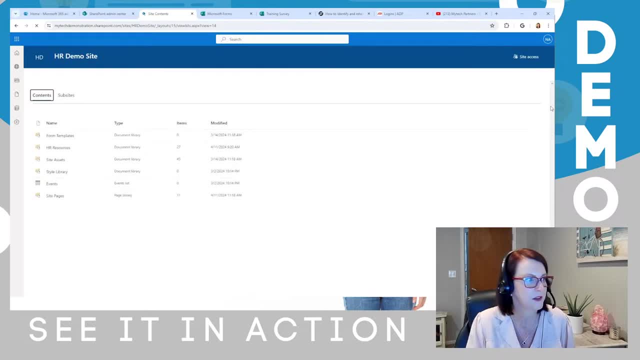 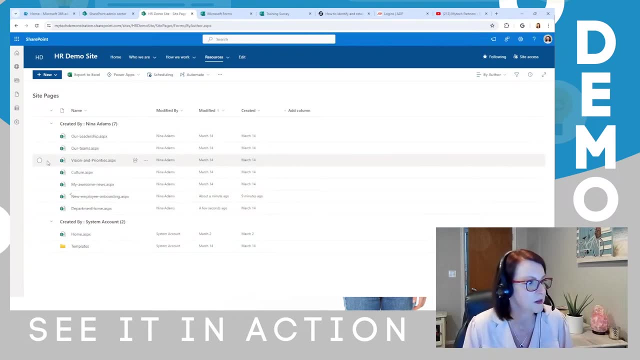 And then I go to site contents, Site pages. Remember, earlier I was saying that there's a library specifically for all of the contents of your site And you'll see, there it is. New employee onboarding. I will say, in the previous session we talked about adding. 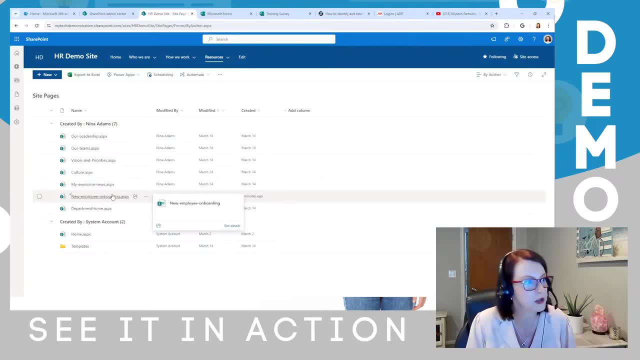 News articles. I will show you again just really quickly how to do that. So news and any additional pages you create all live here in the site contents library. So if you've created news articles and you want to go back and edit them, this is where you would do it as well. 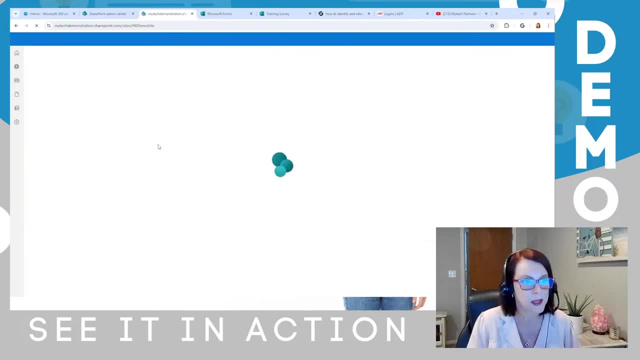 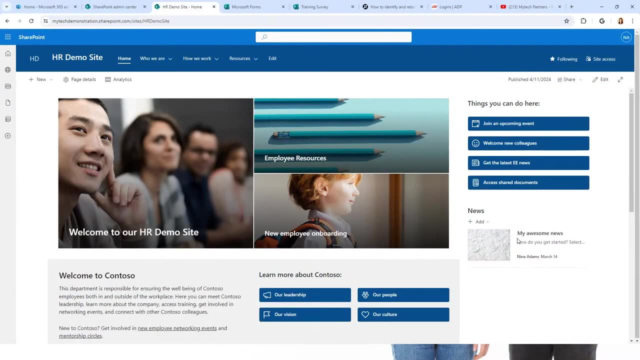 So let me just show that really quickly. I'm going to go back here to home And I think we did create a very brief little news article here. It was called my awesome news in the previous one. I'm going to add one more in there just to show. 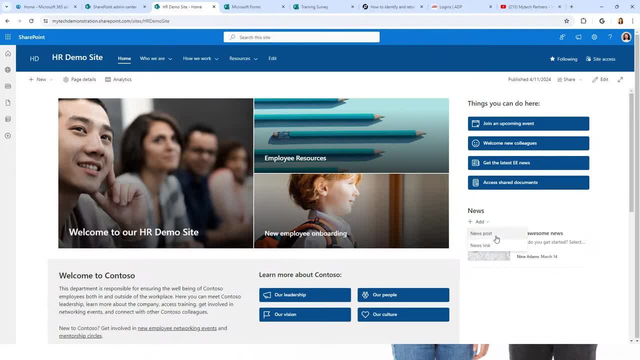 So I'm going to click on add. now I could do a post which is my own news that I've generated, similar to creating the page that I just did, or I could link it to an existing external website. So I just opened one up here. 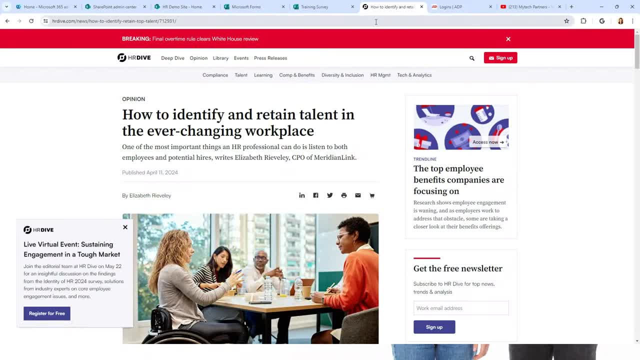 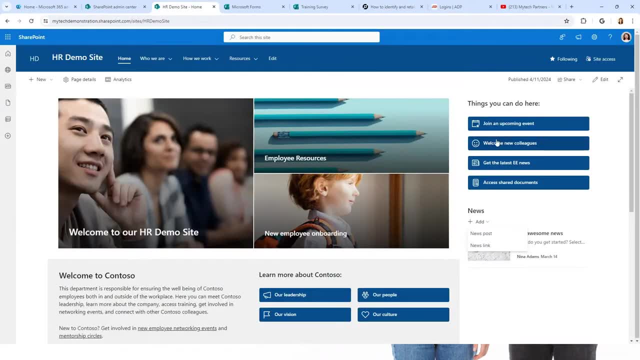 Uh, it's kind of an HR news article on how to identify and retain talent. I'm going to go ahead and copy that URL just to demonstrate how we can link to that news article. So again, click add news link. paste the link in there. 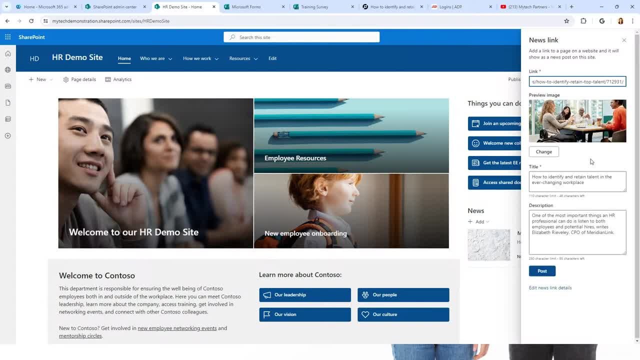 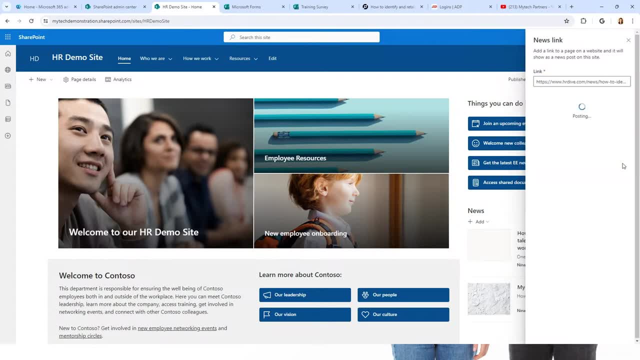 See, it's Uh now connecting to that page. it pulled the picture from that page as well, And I'm going to go ahead and hit post. All right, So I can do my own again, or I can link to other news articles, and we kind of use a combination of the both. 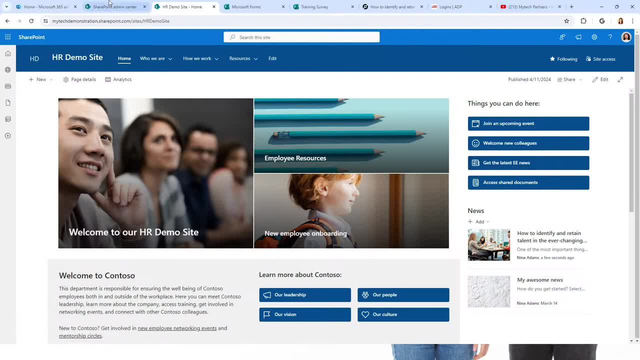 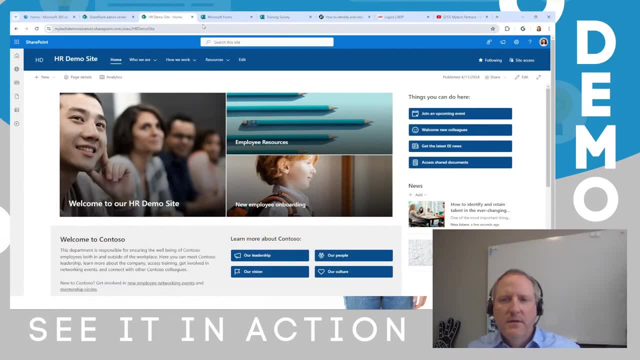 It works really well. And Hey, Nina, can you talk about? um, one of the things that I like about news is how some of the automatic notifications happen when there's like where it can sometimes email folks. Hey, this is what's happened in SharePoint. 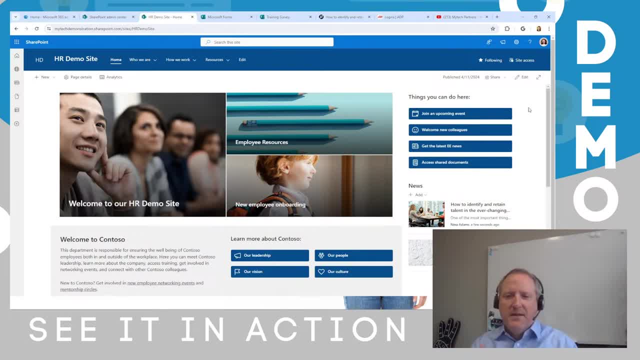 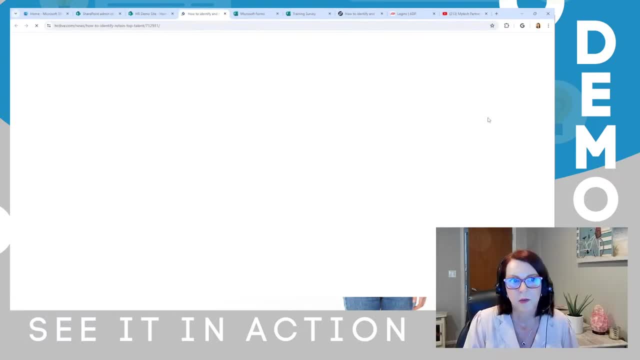 If someone publishes Um cause, posting it doesn't necessarily mean that everyone necessarily knows it's there, unless there's some sort of location. Isn't there some sort of built in notification relative to news? So we can probably dig into that a lot more with Viva connections. 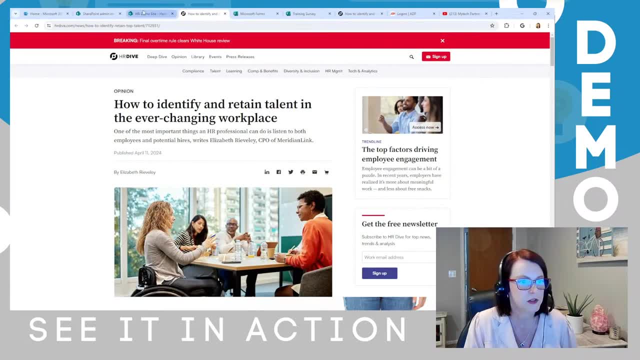 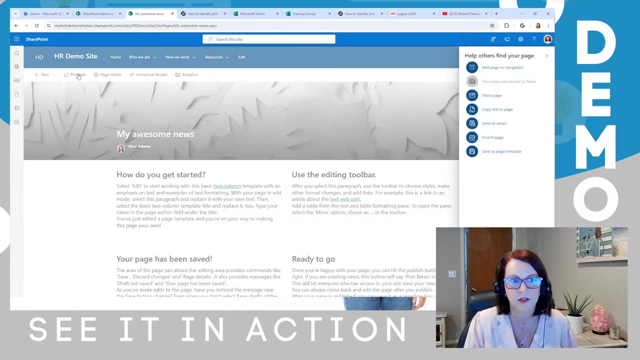 Oh, uh, let me go into this news article here. I will show one other way. Uh, so you can actually promote the news article as well. uh, so that there's uh, you know, and, and you can also encourage people to follow as well. 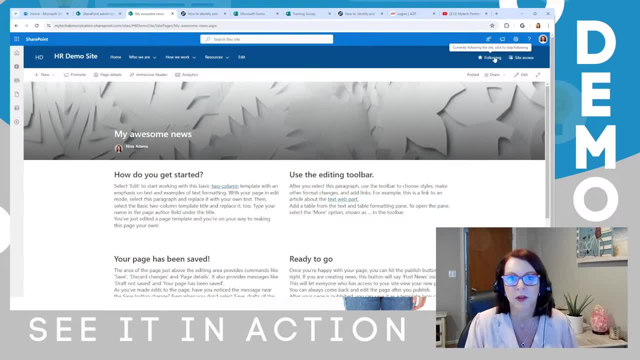 Um, oh, you'll see there's a little following Up here, Um, but when we get into the Viva connections, there's a way that that news will actually be posted, um, you know, across the organization, probably in a better way than what SharePoint on its own will do. 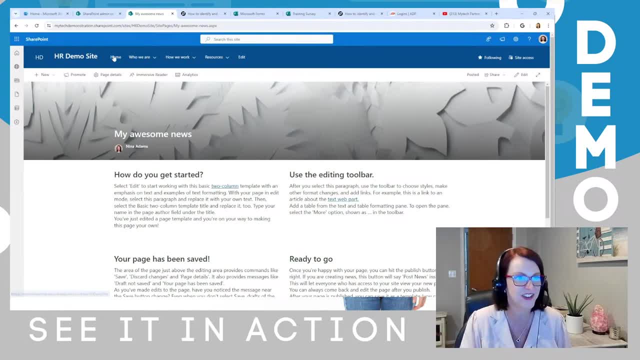 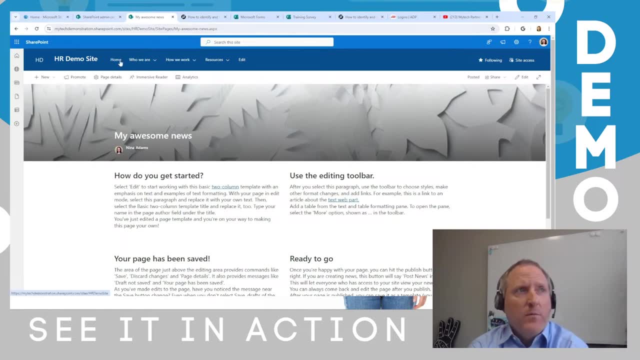 Nice, So I knew there was a way to do it. So sorry to derail. Yeah, no, no, no worries, I think that's a really cool feature because, I mean, I think that that's one of the gaps, I think, that a lot of organizations face. is you feel like, well, I'm missing communication or I'm not? I don't feel like I'm being updated? 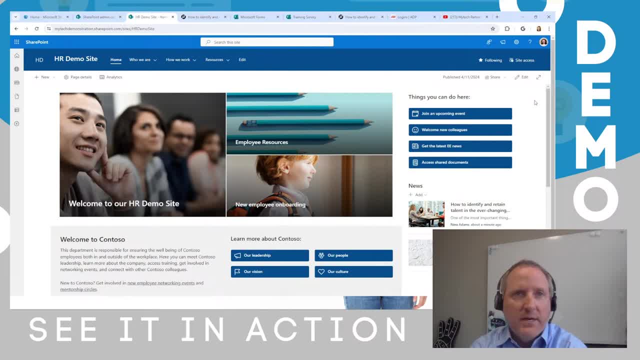 Um, and that's hard across. I mean, every organization Struggles with communication and collaboration, So I just think that that feature um is really powerful to help make sure that everyone in the organization gets notified of things that are really critical to be notified about. 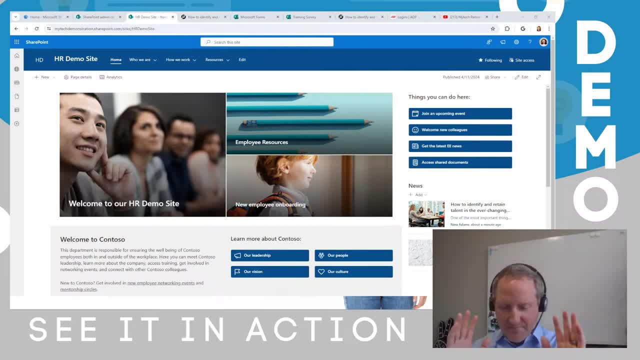 Um, but yet also driving them to the SharePoint portal and all that. So Sorry for the. so here's a foreshadowing. I guess on its own It's okay, But I that I think the real power comes in with leveraging Viva connections. 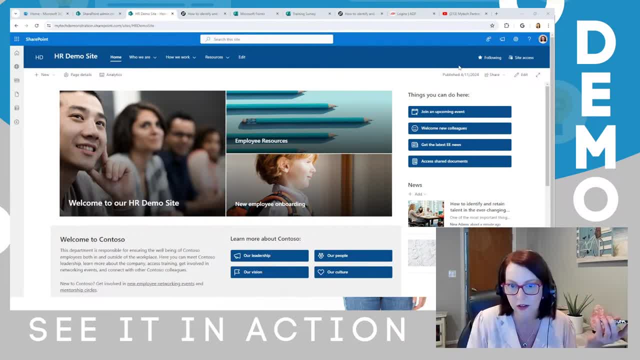 Cause I know you've probably get notified on your phone as well, Mm-hmm, Which I Think is like a really added benefit of of kind of Viva connections and staying on top of some of that news. So yeah, definitely want to touch on that in the next session, for sure. 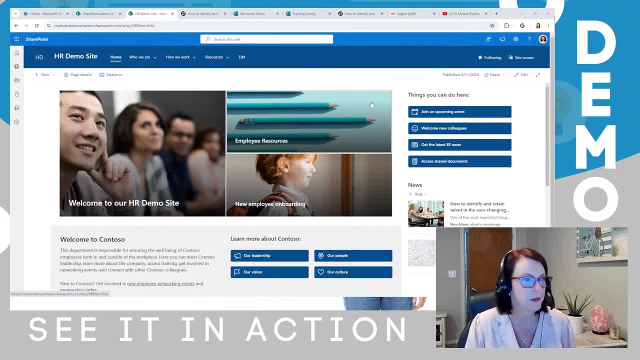 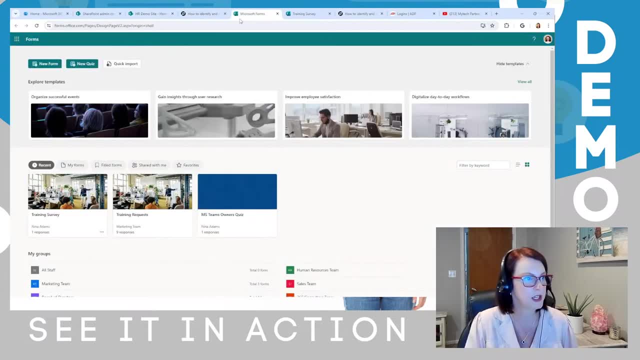 Um, one quick other thing that I wanted to show here on this uh main page while we're here: um, I actually created a form in Microsoft forms, Um, so it's a training survey, um, and I wanted to just that's kind of part of our HR function. 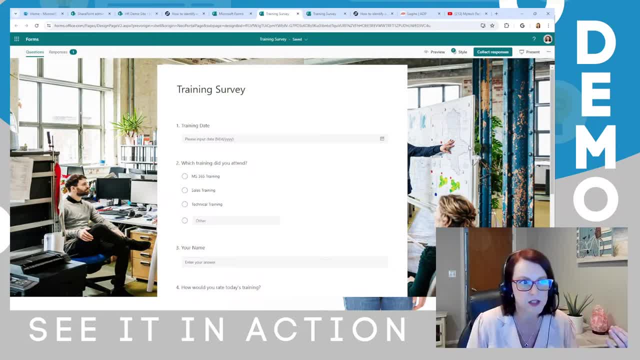 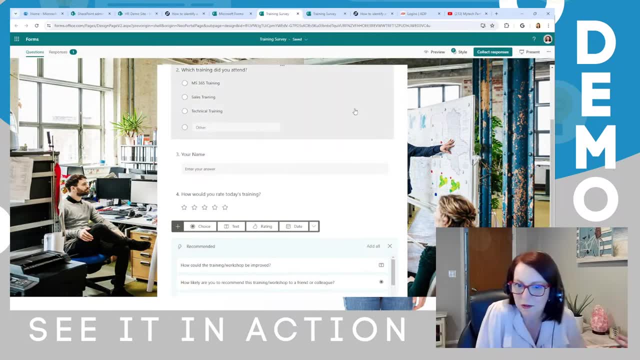 We want to know what training you attended and how would you rate it. Uh, so that's a great example Of how we could utilize forms, but then how do we actually pull that form into SharePoint and how do we use it there, Like you know? is it just a standalone thing, or or can we integrate? 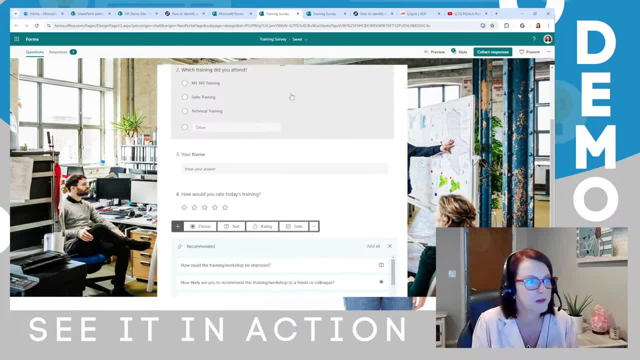 Uh, so I love any kind of integration. you know we just spoke about Viva connections, but, uh, any integration that SharePoint might have with other three- 65 apps to me is always a bonus. Um, so I'm going to just go and edit this page and I want to show you how to actually add a form onto your page. 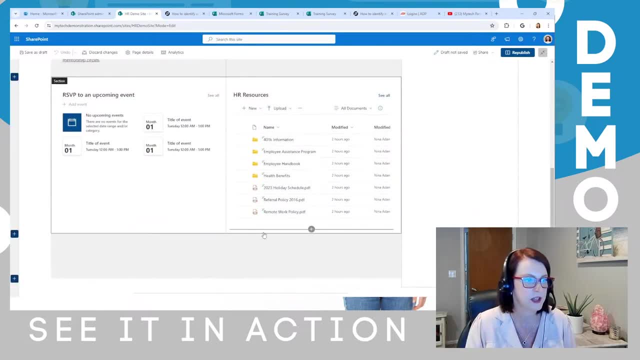 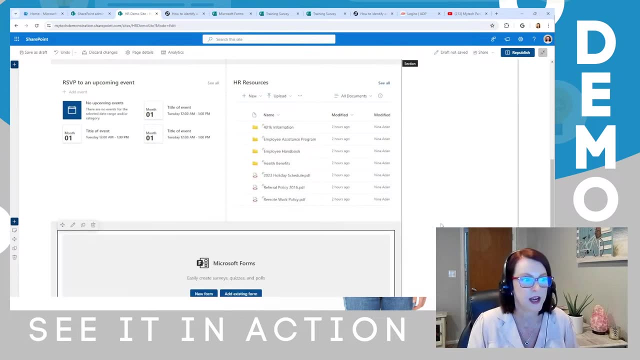 So I'm gonna scroll down here just a little and down here click on the plus sign. Uh, we're going to look for forms specifically. so there we go, and I can either add, create a new form or add an existing form. 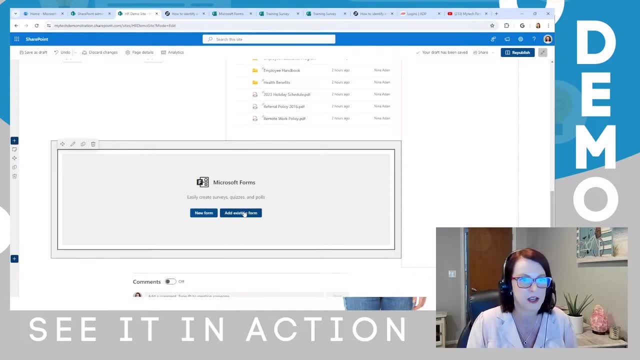 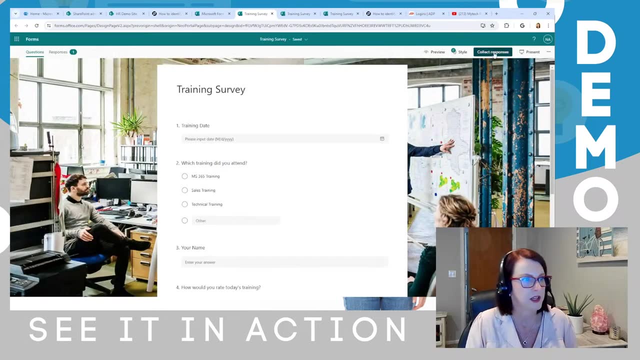 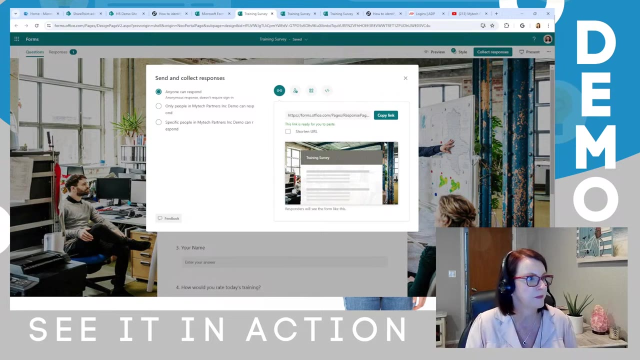 So for the sake of this demo, I've already created it And let me go over here to forms You're going to just click on collect responses, because in here I'd like to get a hold of that link. So I'm going to copy the link and then back on the HR side again. 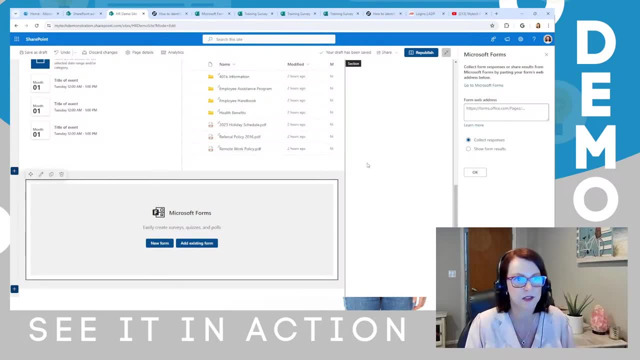 If I can Click on the pencil, I get the little properties window that kind of flies out from the right hand side, and then we're going to paste it in there and click on Okay, right, And there's my training survey. 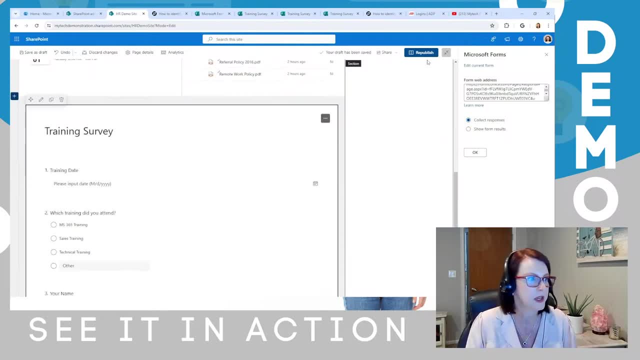 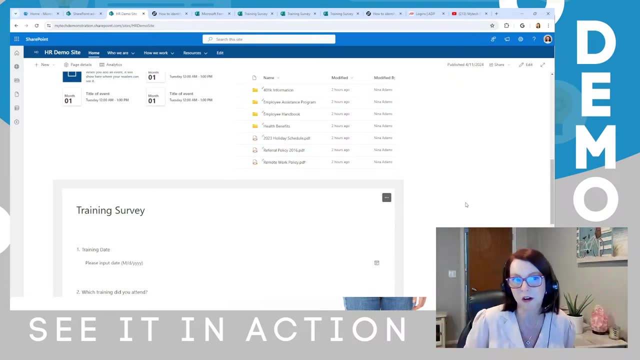 It's embedded on the SharePoint page, um, and click on republish. So again, as I said mentioned earlier, I wouldn't have that page be too long. So potentially what would be better is to actually create another page where you have your survey and then link that. 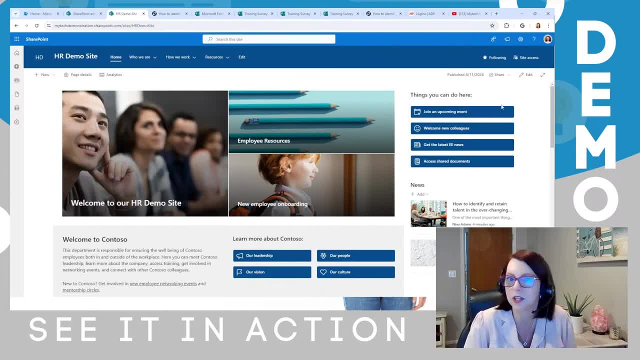 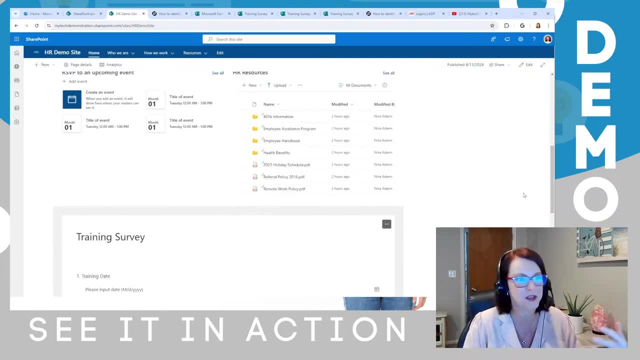 I'm either using these quick links on the right hand side or using your um hero web part, So I'm kind of going against what I just suggested. but in the interest of time, I'm just going to embed it on this homepage, just for you to be able to see how that works. 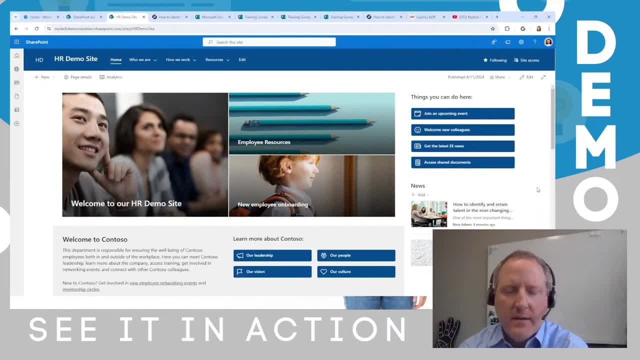 Nate, you look like you have a comment. Well, I was just thinking, yeah, cause I think I think this is a great example too of where, depending on visually and navigation and design, depending on how, um, uh, I don't know, I'm gonna use the word that's coming out in persnickety. you are about that, right? 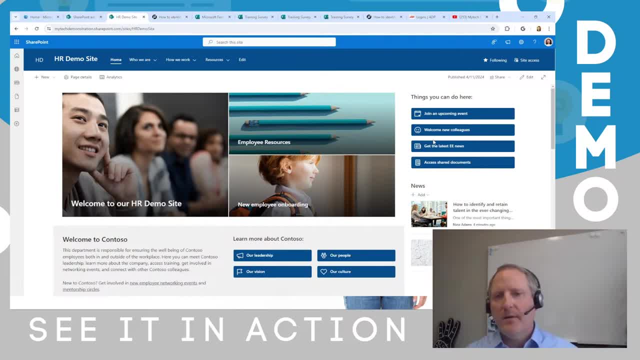 You might choose it, cause like you had some good imagery behind that. So like like where I wonder if you could just quickly illustrate- cause I know it won't take you more than a minute is under the things you can do here- If you could create a button that would then link to that form as opposed to embed it. 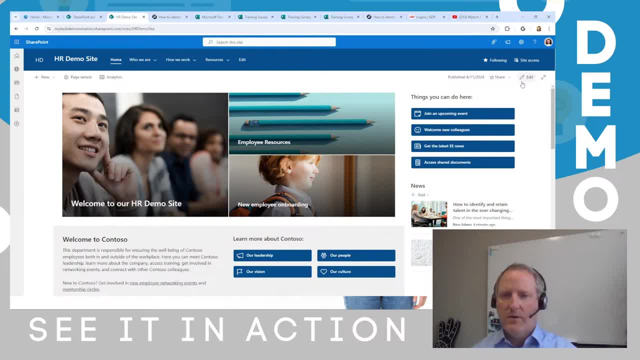 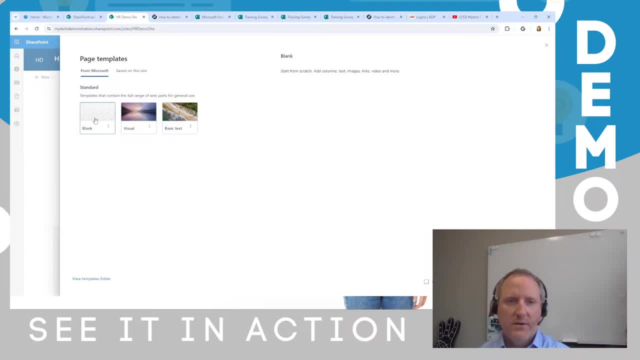 So like just illustrating, like how You could do both um and again. this could be and or, or, both right And or. uh, like you know how you, how you link stuff. So, um, you know, just creating, yeah, just having some sort of a button where you don't have to do a new page. 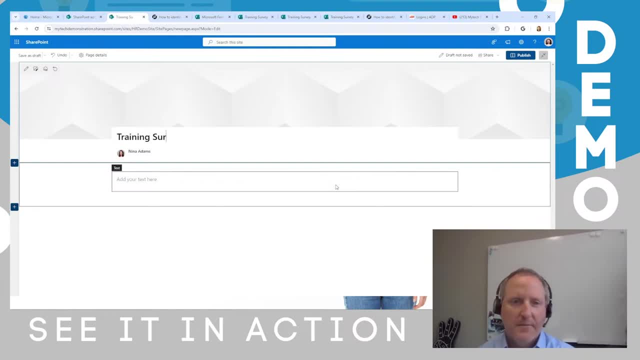 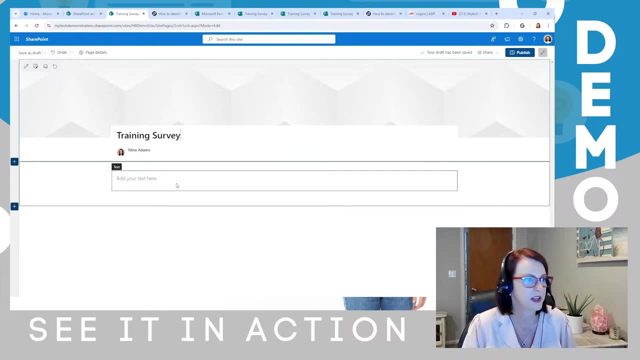 I was just thinking like a, a, a button that would link to it. but either way it works. Yeah, Yeah, And the thing is I just I felt it's kind of better to keep it in the SharePoint site. So it's just yeah, and it's quick enough. 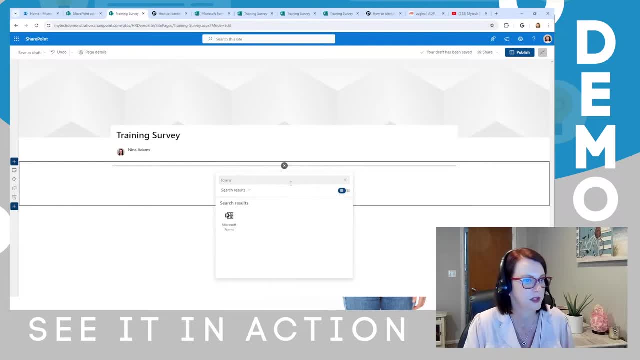 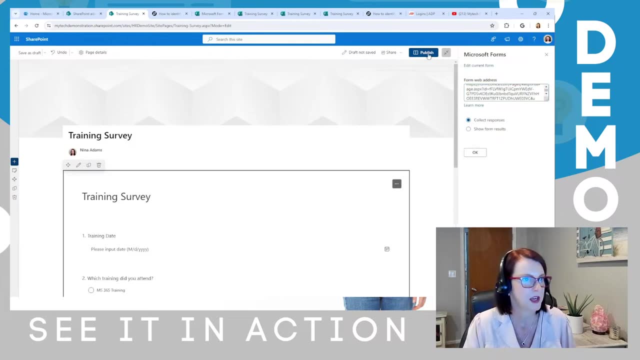 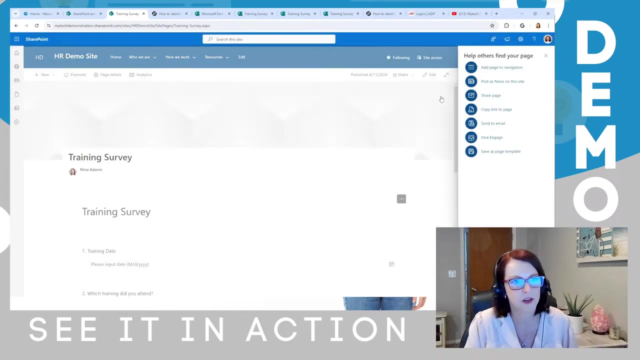 We can do it really quick. forms: There we go: Add an existing Form. I think that link still works. There we go, Uh, click on publish and you could link to the form itself. I just kind of find it looks uh, kind of looks better. um, on a page like this, 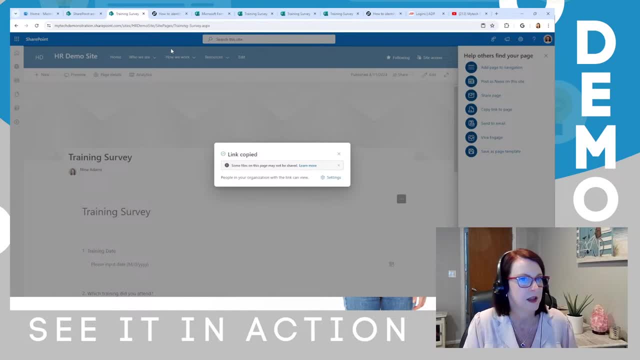 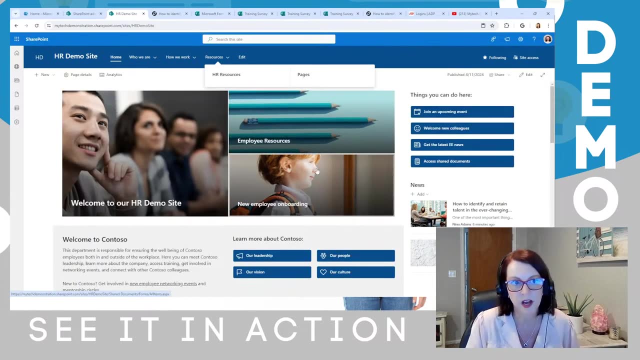 I'm going to copy that link really quickly and go back here to the home. So very similar to how we just did it with a new employee tile. I'm going to click on edit And we're going to Add in a link here. 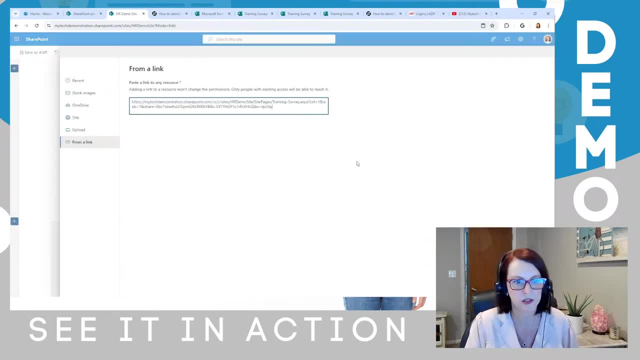 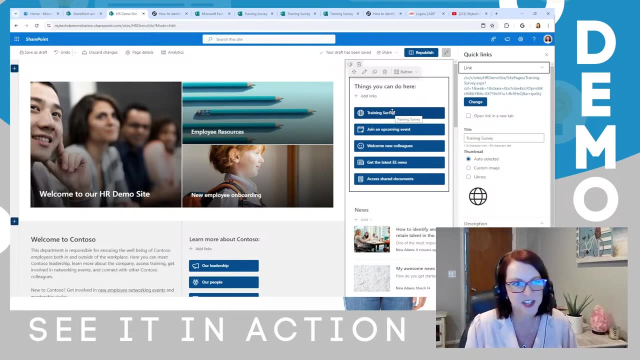 So I'm going to say this is where it should go to this page. Click on add And it even picked up that it's a training survey bonus, So I don't even have to change the title there. Uh, you can also change the order of the links by kind of similar to the web parts, just clicking and dragging. 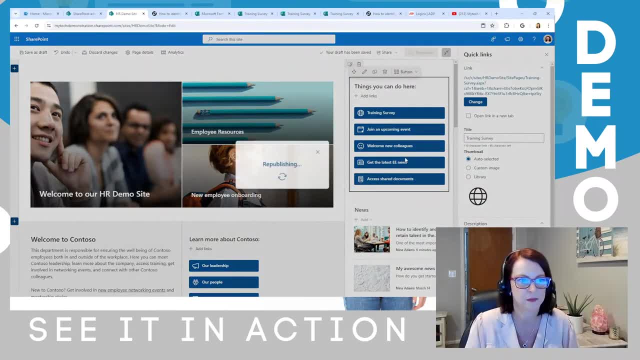 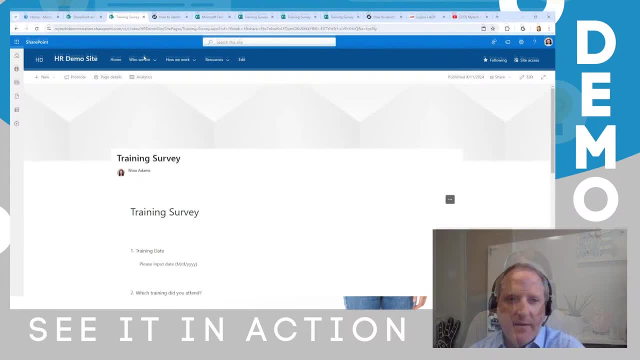 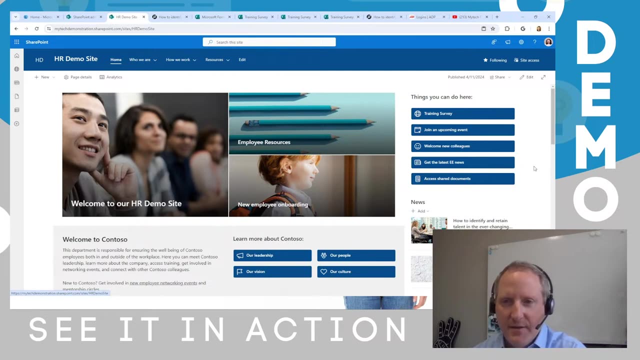 But I think that that looks good and republish And, as always, good to test. Yeah, Yeah, That's just again. I, I, I. What I appreciate about you dynamically just doing that is that again it. it took you probably less than 60 seconds to do that if you already had the form bill. 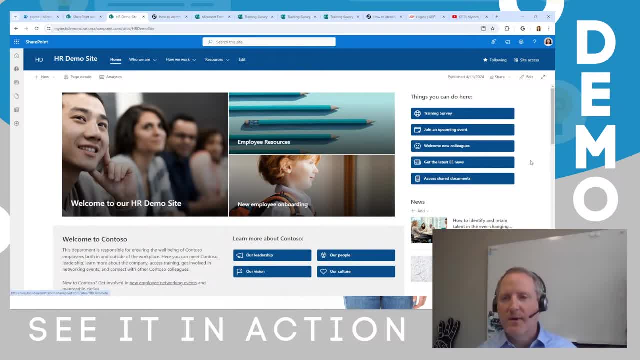 Um, and you know you might have preferences about where, where and how you might want to link things. uh, for just the way it looks for the ease of access or to highlight certain areas, Um, and so it's it. it's not um, it's detailed, but once you learn it it's not that hard right. 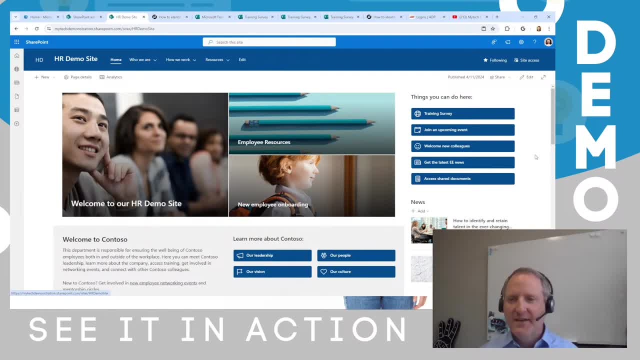 It's. it's not that difficult to do. Like like Nina said before, it's not code- you know I'm doing that kind of stuff- But it is thinking about the layout and thinking about your audience, thinking about ease of access. 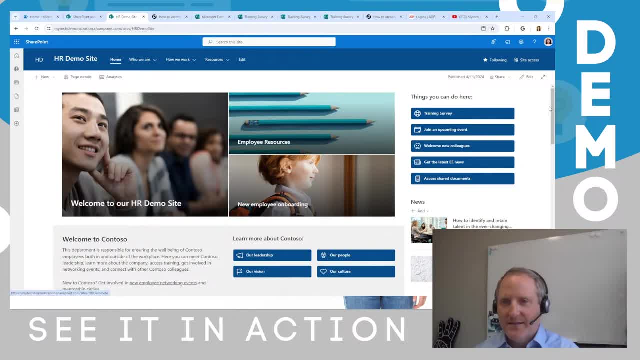 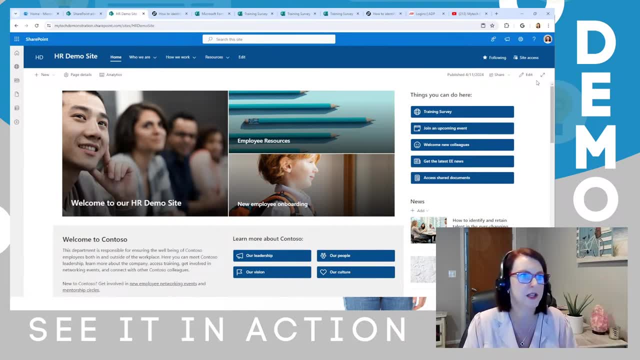 It does. That's probably the harder part of it than than actually making the clicks to to get it to work. Yeah, And if I can give any suggestion here with like the different web parts and what they do is create a test site for yourself and just go and play. 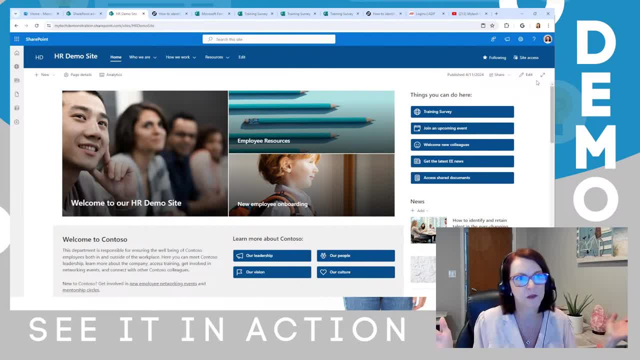 Like there's unfortunately not enough time to go through every single web part and exactly what they do. but um, that, in my experience, is the best way to figure it out. It's just to play. just Add things to your test page, see what it does. uh, you know, try it out. 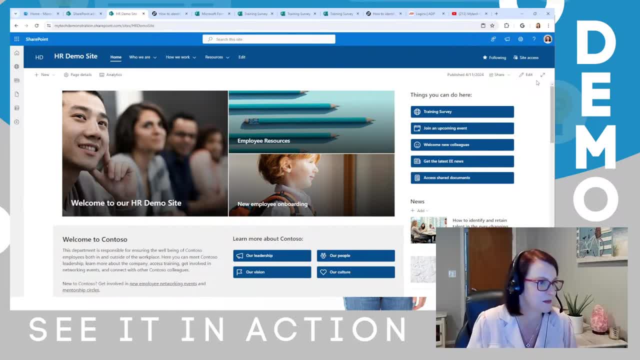 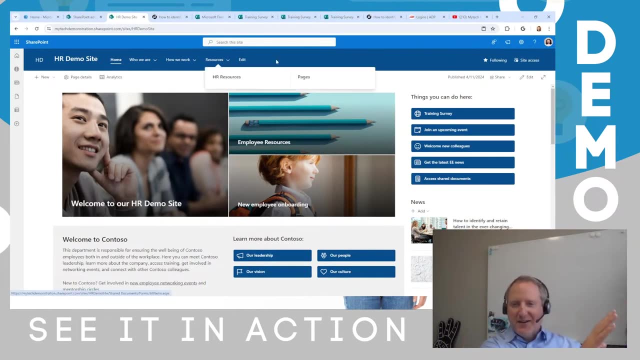 That that really is the best way to learn, as with most things Well, and the other thing about that too- and I know we touched on this, I think, last session- but to re reinforce you, you can create a site Without and play and do all the things that Nina just talked about without having it publicly available to everyone in the organization. 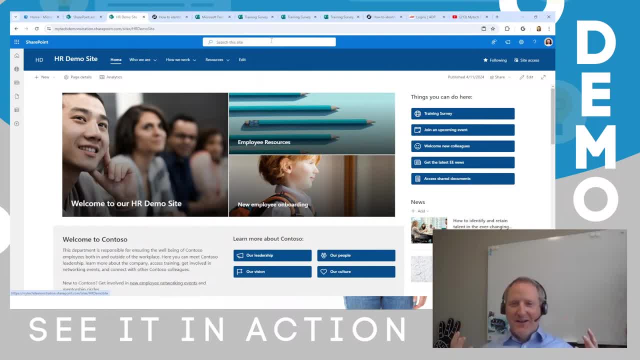 Right, So you don't have to worry about everyone seeing your playground, if you will, if you're just trying to make uh, just trying to figure stuff out Like Yeah, Yeah, You don't have to let people, other people have access to it in the organization until or, if you want to. 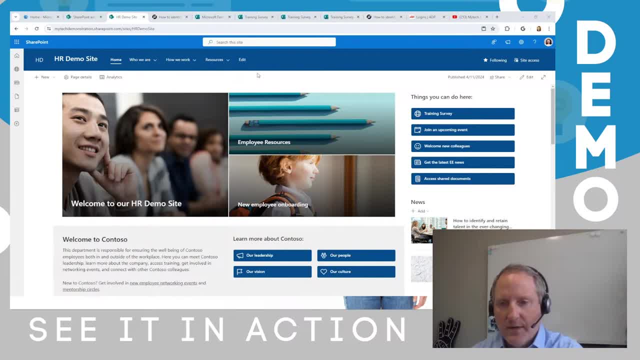 And so if you, as long as you're, have the ability to create a SharePoint site, So, um, that's that's something that I know people have have worried about- And also if you have an existing SharePoint infrastructure, the other way this works is you can build out site by site, page by page, the infrastructure before the an alternate uh um sites or alternate structure, without giving everyone access to it. 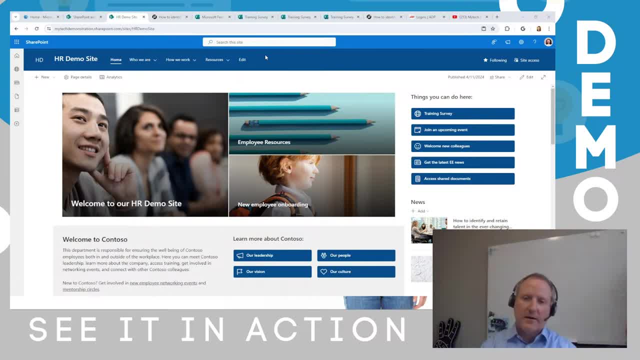 Then, when you're ready, you can then kind of switch everybody over to it. So that's something Nina is going to talk about next time as well. Um, pulling the pulling the hub sites together. but sorry, I feel like I'm derailing you a little bit, Nina. 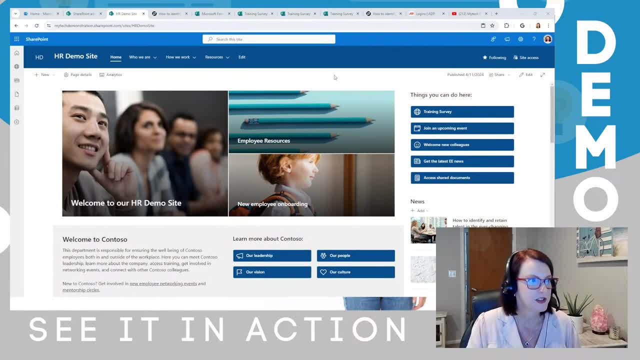 I want to make sure you get through everything you wanted to cover today, No worries. Last thing with the time remaining that you want to touch on is just the navigation, and we are going to dig into navigation a whole lot more in the next session as we kind of bring the collective sites together. but just a really quick uh, like the how to hear on, like your site navigation. 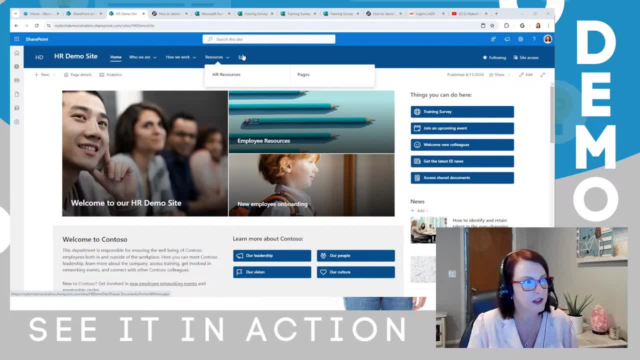 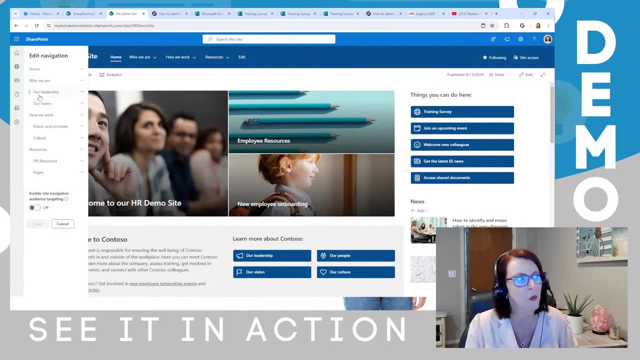 Um, so this is the edit button in the middle, not the one on the right. So we're going to click there on edit. Uh, and for those of you familiar with OneNote and how you have pages and sub pages, this kind of acts in the same way. 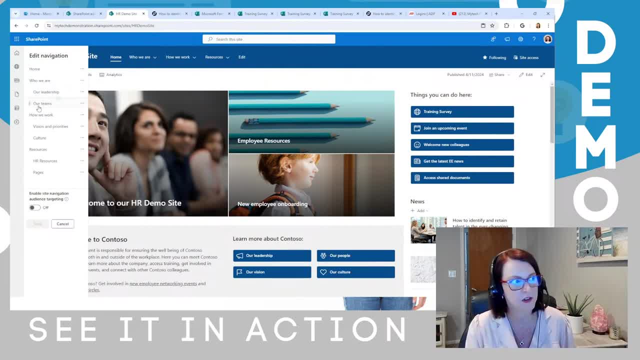 So these, uh, the headings that are very left aligned here, are really these top level headings, Um, and then the kind of sub sub headings underneath them are the ones that kind of cascade into um, the ones underneath it, Um, how do we add it? 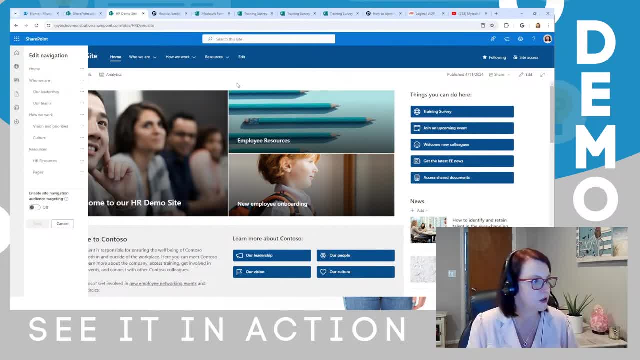 So, uh, let's say this page that we just created the survey. um, I'm going to actually remove the. how we work, We don't need this for this particular site. So I'm going to click on the- the uh little breadcrumbs there- and just 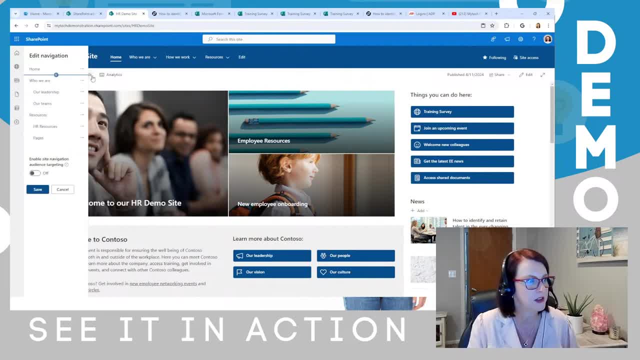 Remove it completely. Same thing with who we are. I'm going to click there and say remove, but I do want them to fill out a survey for me, So I'm going to click on. plus, I have two options there to do a link, which is obviously the URL, or a label. 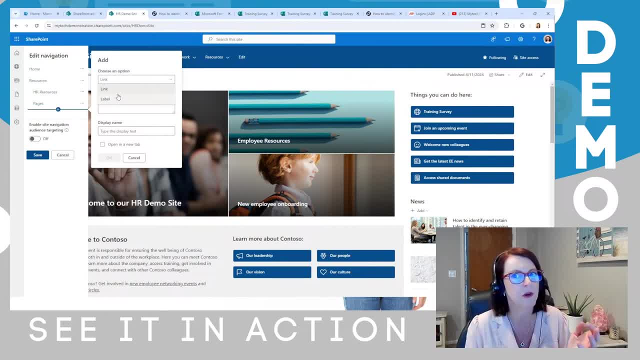 And I'll talk a little bit more about labels in the next session as well, because it's a great way to use uh to set up your navigation, to see what it potentially will look like without maybe having those pages ready to go yet. 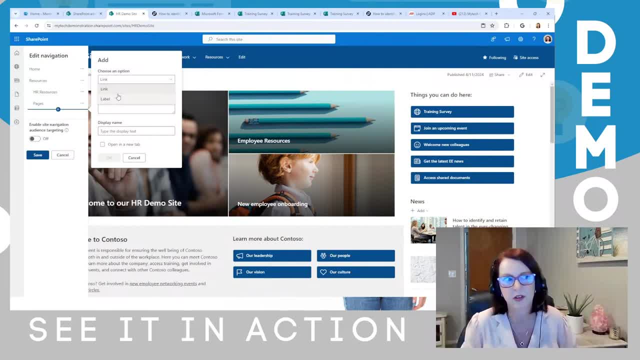 But you do want to kind of wireframe it, if you will. Um, and labels are a great way to do that. But for this one we have a link. I'm going to put in the address there and I'm going to say, uh, employee survey and click on. 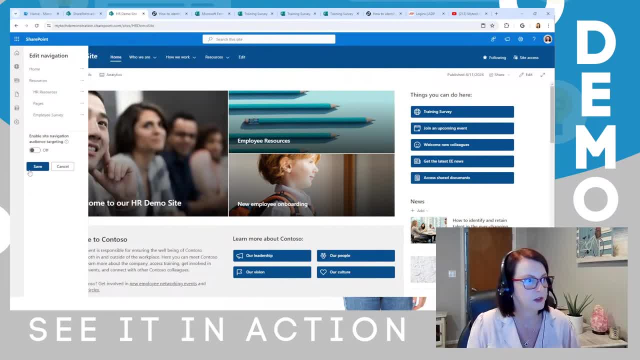 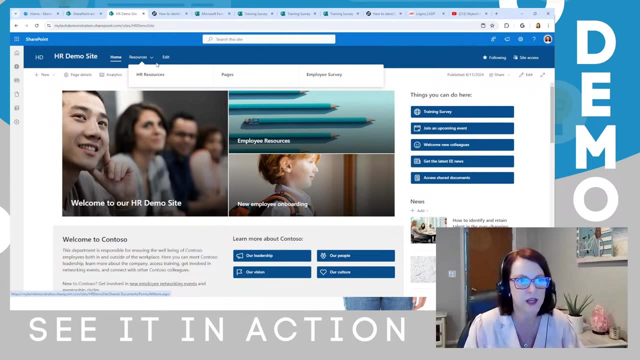 Okay, So right now, if I click on save, you'll see how that's changed. Employee survey now lives underneath um resources. Um, so you'll see. with the navigation this is currently set to mega menus, So I want this to just look like a very normal cascading menu. 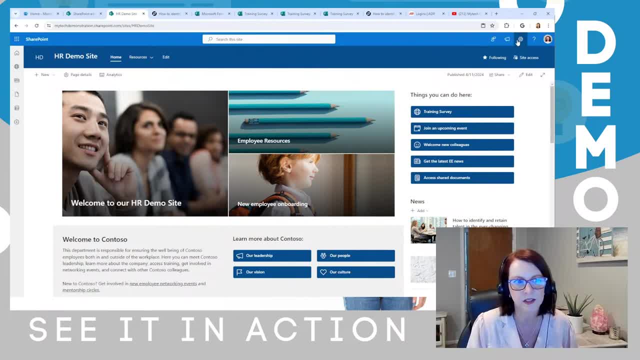 Uh, just a quick uh refresh on how to do that. Just settings change the look. uh, my uh, oh sorry. Navigation. So at the moment it's set to a mega menu. I'm just going to change it to a normal cascading menu. 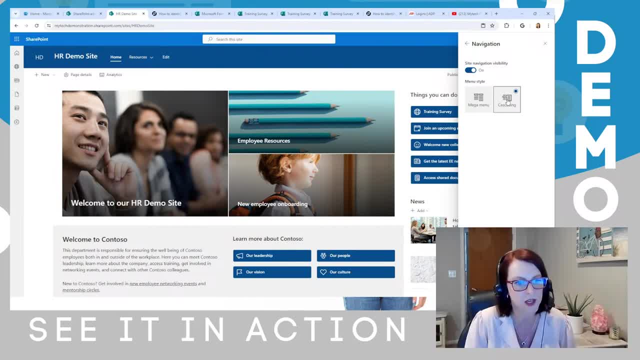 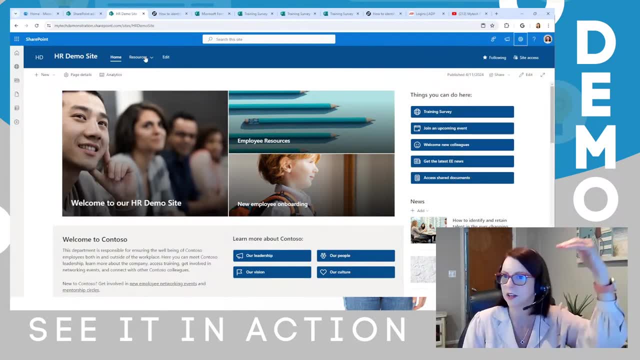 We don't have that many links that we need a mega menu, So just a normal cascading menu and close out of there. So this is what that would look like, So more of a kind of just a normal dropdown menu. Um, but let's say I I don't actually want employee survey to be a part of resources. 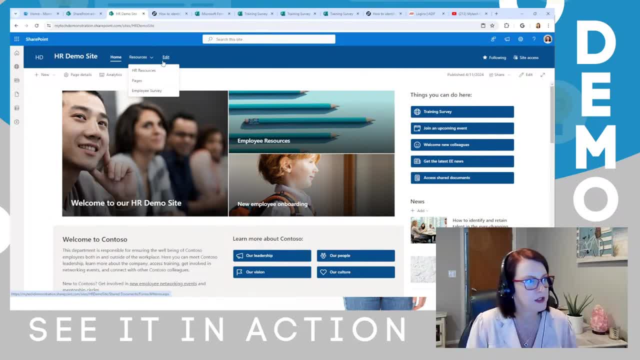 I want it to be. I want it to be like a standalone link. So if I go back into edit, what I'm going to do is click on the breadcrumbs and then say, promote it, so that it's kind of a main link. 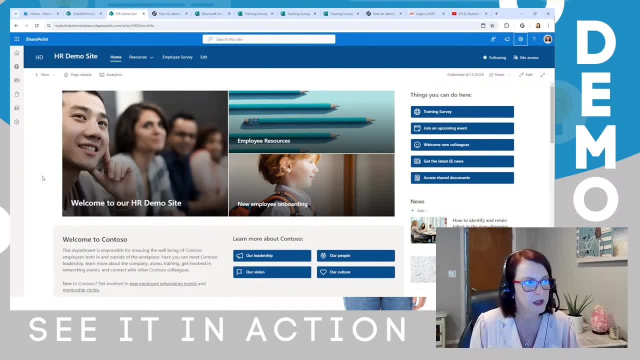 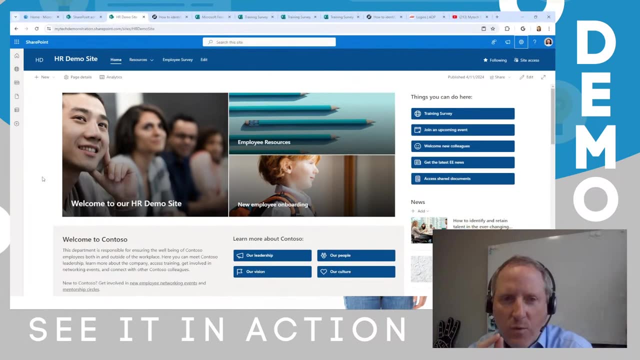 So if I click on save there you'll see that it'll pop up as its own link. So some of those best practices and things around navigation, especially as we start looking at global or hub navigation, we'll kind of discuss those in the next session a little bit more. but that's just a little quick intro onto site navigation. 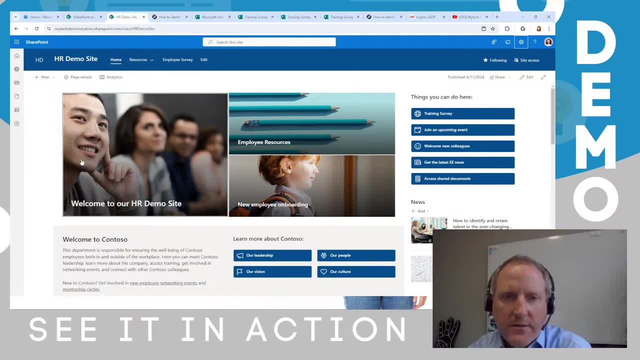 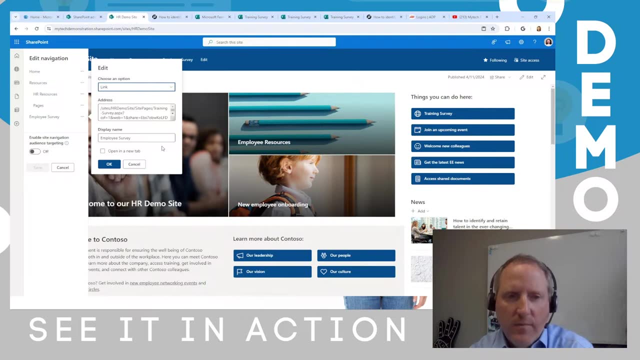 Nina, could you show one more thing, Cause you were right there? Yep, So one of the things that I like to call it out to is: um, and click on the edit for employee survey, where you click on the little breadcrumbs. um, one of the options, just the edit, the edit there. um, one of the options on these pages. notice there's a little checkbox that says open a new tab, like you may want to. you know this is like: uh, you know you can go to a public websites, right? 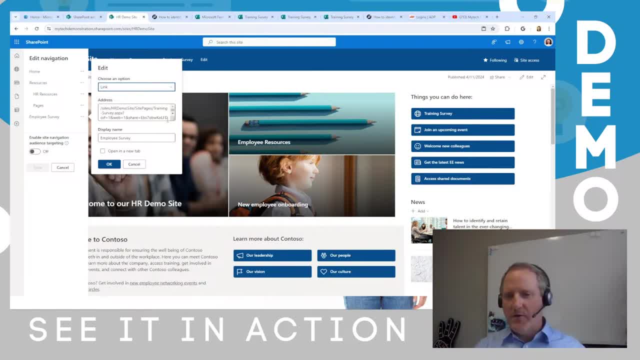 And sometimes you click on a link and it- uh, it's hard. It takes you away from where you are, but you could choose whether or not it opens when you, when somebody clicks on it, if it opens a new tab or within the same tab. 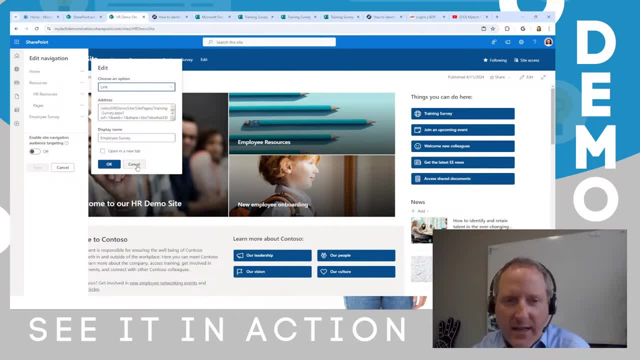 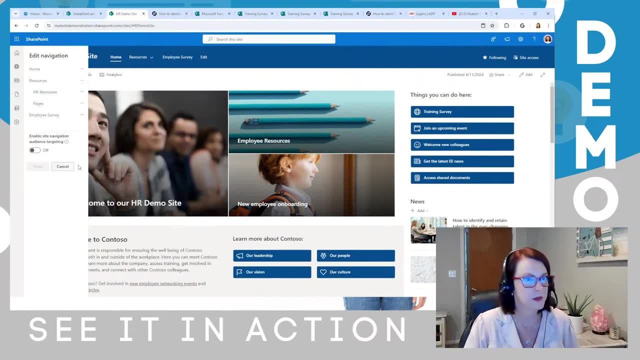 Um, so again, I'm not saying either one's right or wrong, It's just I like to show that's a little spot that you can uh customize on each basically uh link uh page. Yeah, And I actually let me demonstrate that just really quickly before we wrap up here. 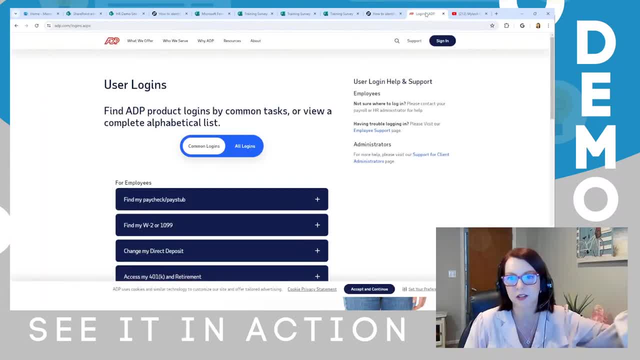 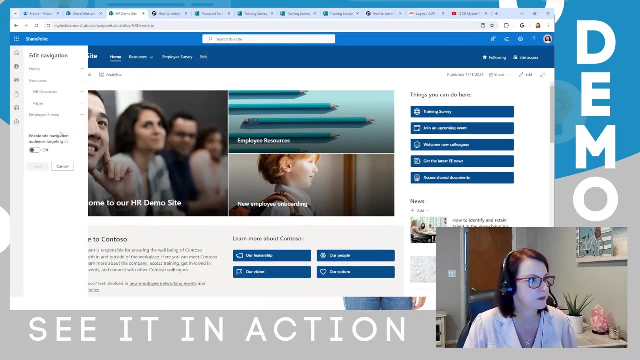 So a great use case for HR is there's usually external HR systems that we want to create shortcuts to, So ADP or whatever your HR system is, and we want to make it really quick and easy for people to get there. So I'm going to just use that URL and on the HR site I'm going to add it in here: um, the link to ADP. 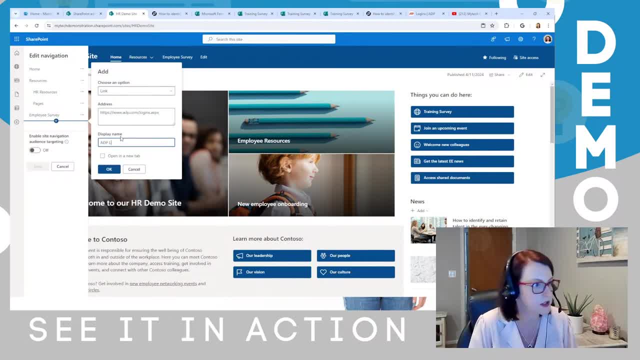 Okay, And we're going to say ADP or whatever your HR system is, ADP, log in. Um and again, as Nate said, if it's external, I always like to make it open up in a new tab. Otherwise it just kind of gets confusing and people are like: where did my SharePoint go? 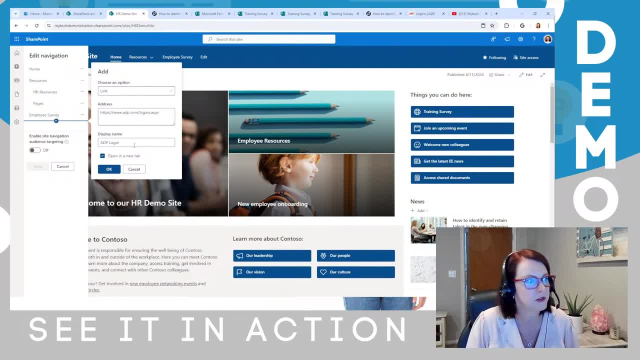 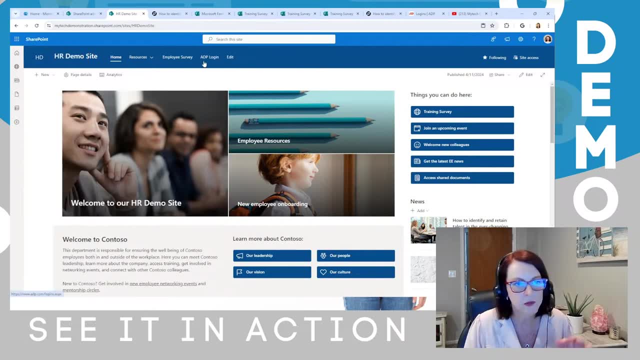 Uh, so that's a good uh, a good best practice for external, So I'm going to click on okay And click on save. Um, one last thing I just want to note here is that sometimes you'll see that there's a little bit of duplication when it comes to uh, setting up navigation. 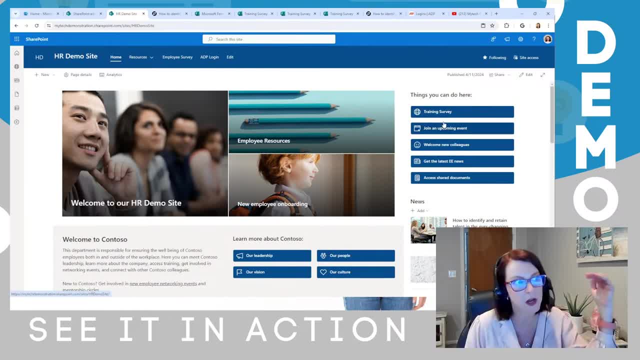 So you may have The ADP log in here as well as at the top. or maybe there's some overlap here with the hero web pod. Um, don't worry about that too much. in my experience, uh, different people look for links in different places. 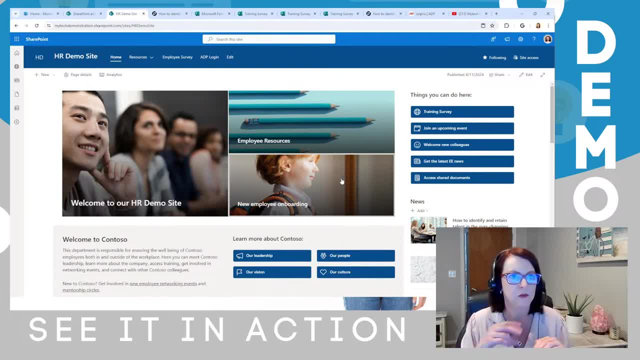 And so I do tend to have a little bit of overlap with that And we'll we'll look at that in more detail as well in that kind of how we set it up for you know, globally as well. But you know, some people are very visual and you know they see that hero web pod first. other people tend to look for, you know, links at the top. 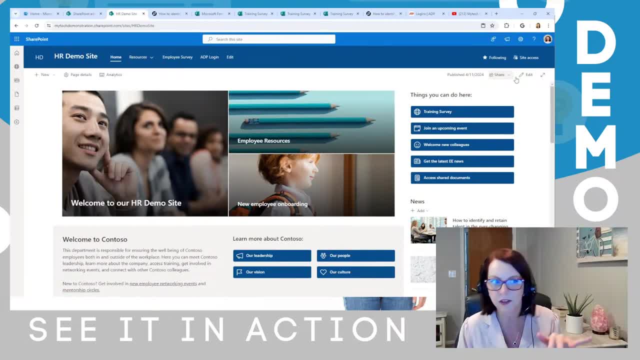 Like I do, or maybe, as they're kind of navigating in the site itself, they may be looking for it in quick links. So just a quick note there. if you do find you're thinking where should I put it to to the link: be here, here or here, um, try it out. 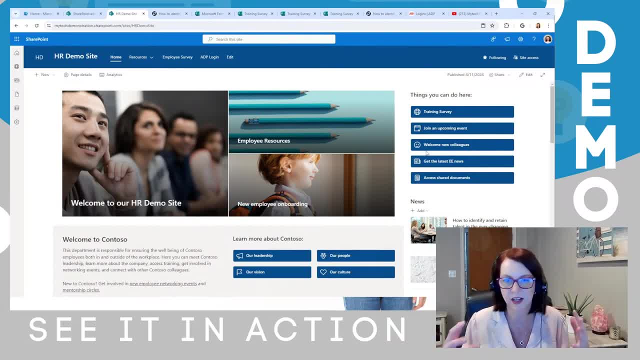 Uh, I usually recommend having a small group of people that are kind of act as your focus group, um, and have them test it for you and say, Hey, you know, I really struggled to find it. or Hey, this really works well. 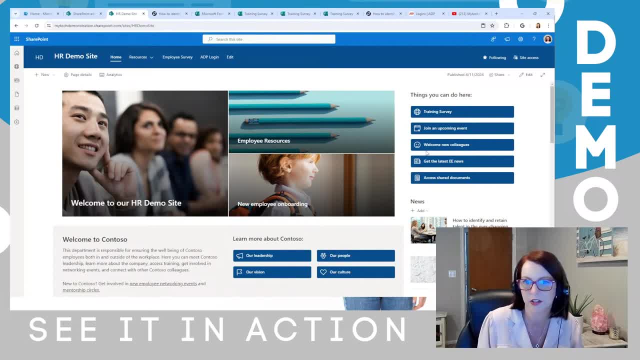 The way that you've said it. I was always good to test it out, So that's kind of my feeling. My final note there before: um, uh, we maybe opened this up to Q and a. Yeah, Nina, thank you. 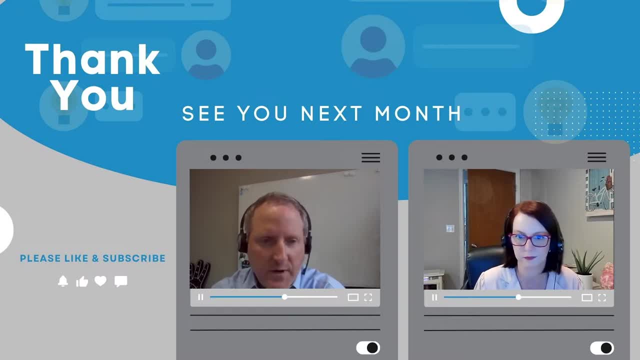 So, uh, look, everyone, thanks for watching this session. We're- we try to break these down into bite-sized chunks, uh, relative to um, all that is, And we, we're. we're not even getting into everything, of course, but these are some of the high-level things that we really try and work on that. 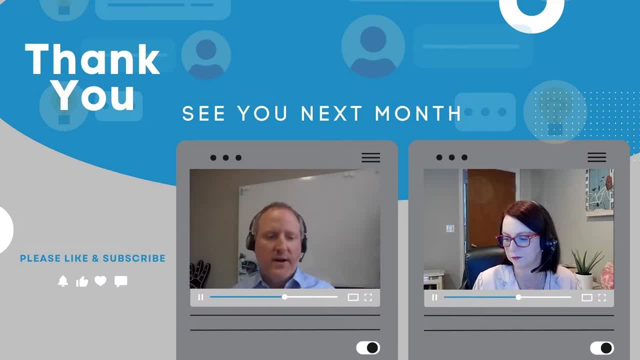 If you're considered, if this is something you're doing as an organization. you're trying to drive adoption, uh, and you've, you've, spent some time and effort maybe making sure you're, Uh, your teams are set right. 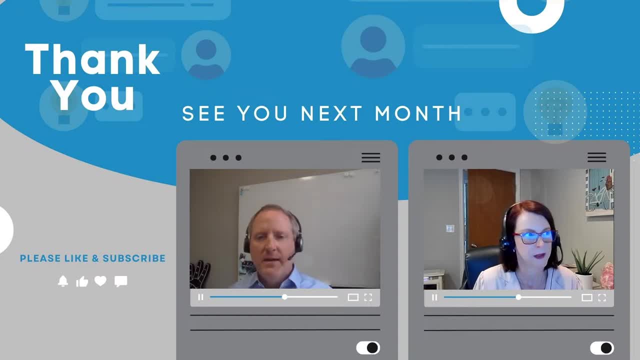 And your SharePoint sites are set right, Or at least the conceptually design of them. This is the last piece. right Is really putting it all together into SharePoint, making it easy for your team to access, easy for your team to search, easy for you, as different departments, to communicate out to your, to out your organization and your and your team based on things that you might want to communicate. 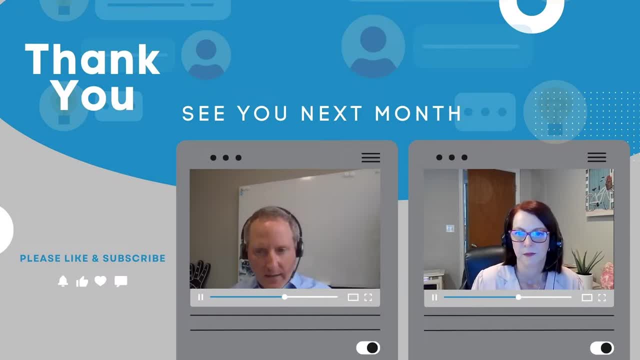 So, uh, thanks for watching session eight. uh again, session nine: uh, next month we're actually going to be getting into taking, imagine you have Uh, five of these different sites. may, I don't know- picking a random number, but it could be 10, it could be a hundred. uh, probably not a hundred, but but maybe you would. I don't know. 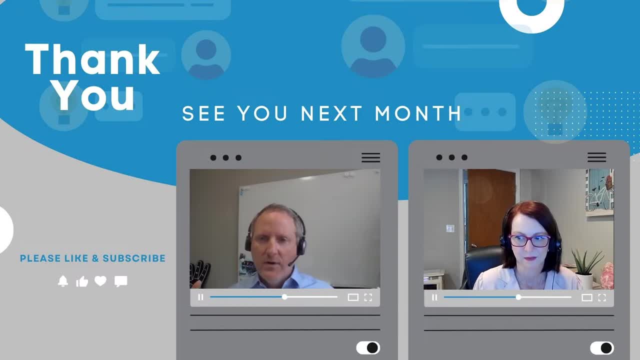 Um, but, but let's say you have several different department sites. Well, how do you pull those all together into a more global uh SharePoint hub or portal or intranet uh that then allows you to connect it into teams and make it easy for your team to access and intuitive for your team to access?